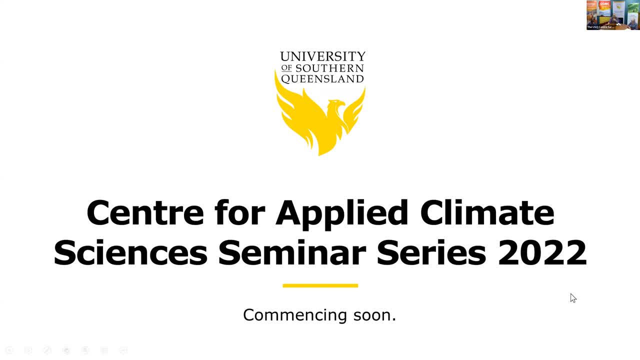 Good morning everybody and welcome to the Centre for Applied Climate Sciences seminar series for 2022.. Today we have Professor Jacqui Croke from the University College of Dublin presenting on the topic of using paleoclimate data to better inform hydroclimate variability and the benefits to the water industry. My name is Kate Riordan-Smith and I'm one of the research. 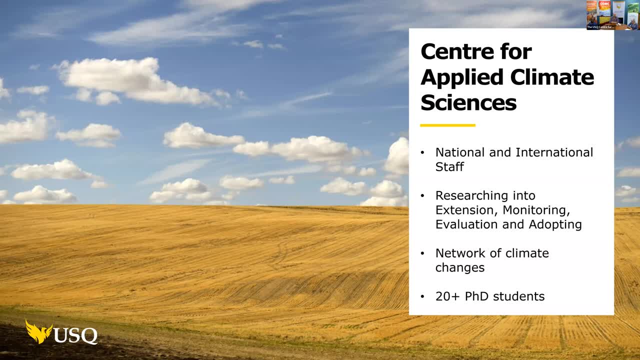 fellows here at the Centre for Applied Climate Sciences. Our centre is based at the University of Southern Queensland. We have approximately 22 staff in southeast Queensland, Melbourne and the UK. We conduct research, including inter-extension monitoring, evaluation and adoption, to help people manage some of the risks they face from climate variability. 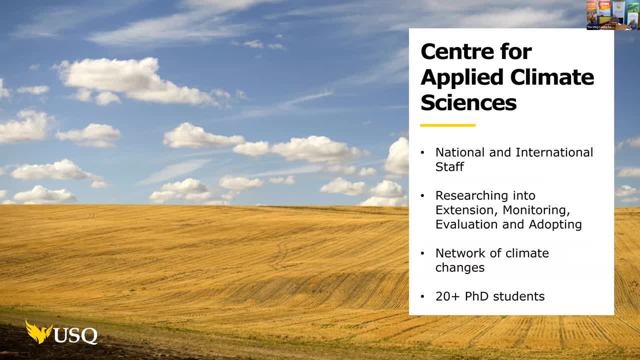 and climate change and to benefit from associated opportunities. We're also a research fellow at the Centre for Applied Climate Sciences. Our research We also employ a network of 16 climate mates located right across Northern Australia who act as champions in the use of meteorological and climate science in decision making. 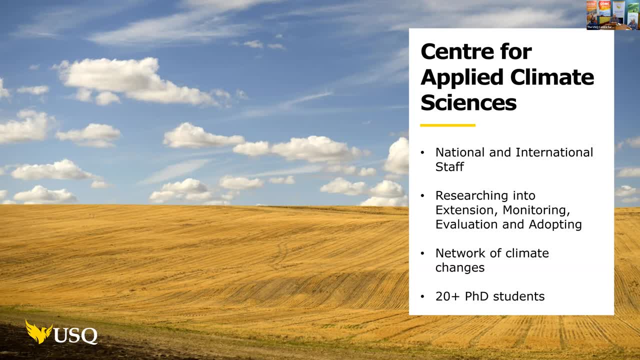 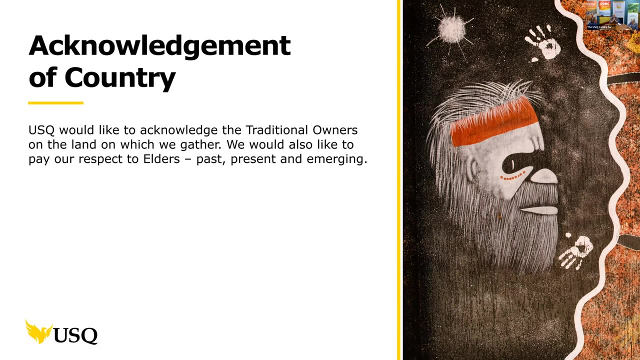 In addition, we have some 20 PhD students located both here in Australia and internationally, particularly in Southeast and Southern Asia. USQ acknowledges the traditional owners of the lands on which we gather. We pay our respects to elders, past, present and emerging. 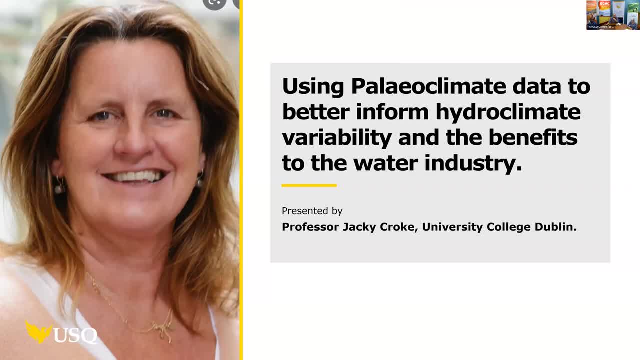 So our speaker today will be Jacqui Croke. Jacqui is a professor in the School of Geography at the University College Dublin. Her research interests lie in fluvial geomorphology, environmental change and landscape response over timescales ranging from the Cotonou. 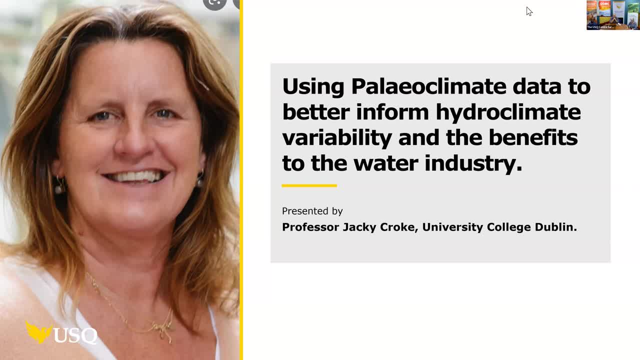 Ternary 2.5 million years ago to the more recent Anthropocene. Key projects include the Big Flood Project, an Australian Research Council funded project involving industry and research partnerships that defined landscape response to extreme flood events in Southeast Queensland, Australia. She is also involved in the Drought and Climate Adaptation Programme project. 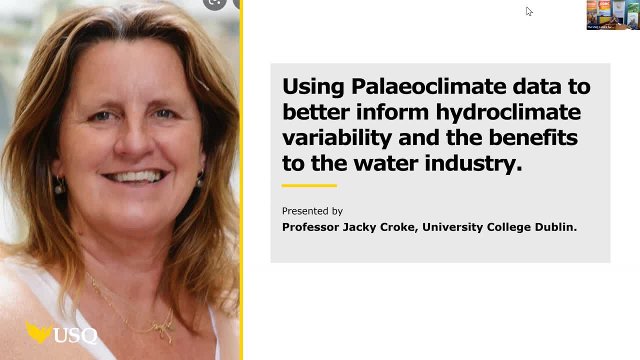 Paleoclimate for water security uses. She is also involved in the. I think you will have all read her abstract, so it's my pleasure now to invite Jacqui to speak, following which we'll have 15 minutes for the Q&A session. 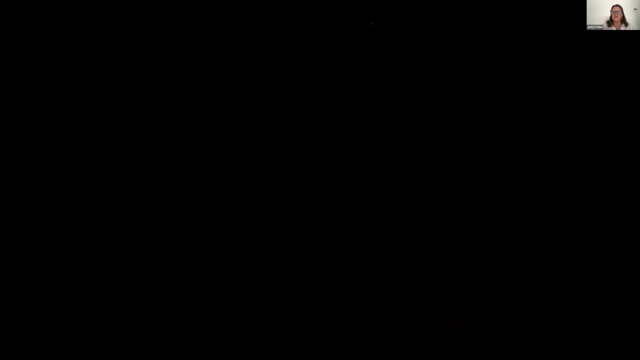 If you have any questions, please enter them into the Q&A on your screen. I'll hand over now to Jacqui. Thanks, Jacqui. I think we've got about 15 minutes to talk to the group today. It's a pleasure to be here. 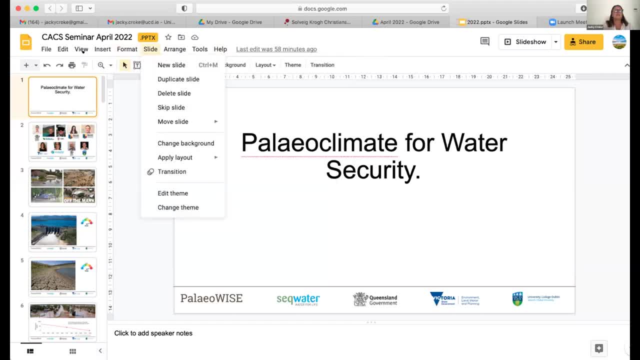 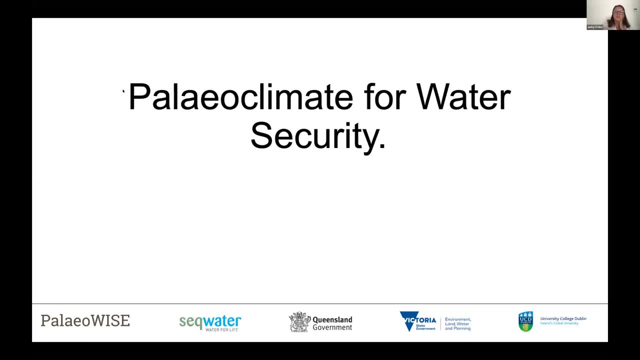 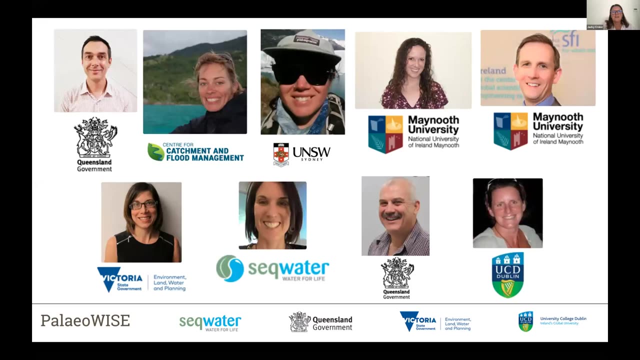 I'll just put this in Yes slideshow. Here we are. As Catherine mentioned, the project that I'm working on, Paleoclimate for Water Security. it's part of a reasonably large team of us here between Queensland and Ireland and Victoria. 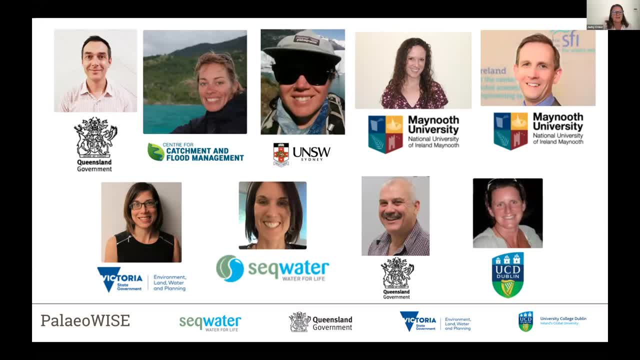 It sounds like a rather eclectic combination of people, But I've spent over 30 years actually in Australia working on various projects, as Catherine mentioned some of them there. Perhaps the most relevant is the big flood project which came into being after the 2011 Queensland floods in the Lockyer Valley and surrounding areas. 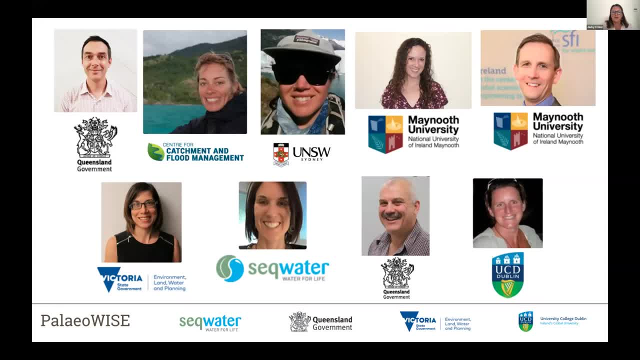 And I'll put up a link to that website. But first of all just to acknowledge our collaborators here: John Vitolsky from the Queensland Government, Kate Hughes, other people there SEQ Water And, as Catherine mentioned, this is a DCAP-funded project as well. 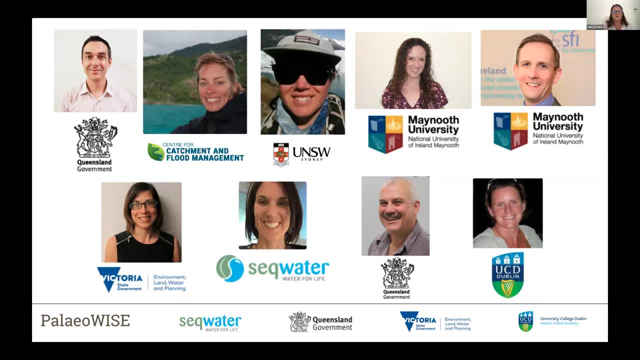 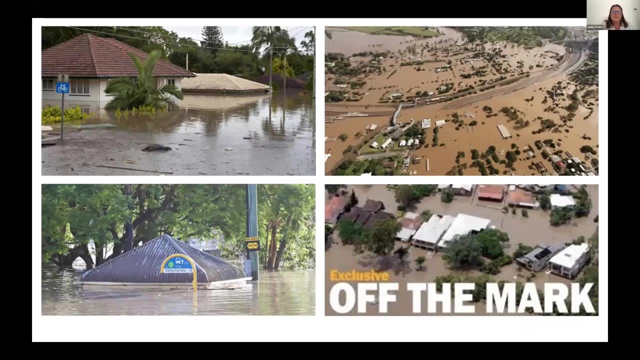 And Ramona Della Posa from formerly DES, but also the Victorian Government and my collaborators back in Dublin. So, by all means, I'm talking today about a large body of work, but tremendous team effort here across continents, really. So the context I guess for this work really did start with that 2011 extreme flood event. 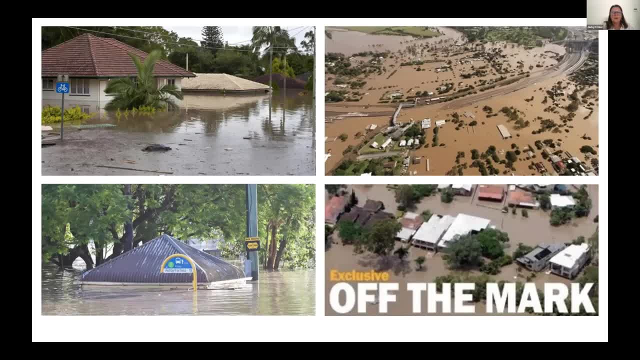 And I know those of us in Queensland have just been through Queensland And Northern New South Wales- in fact, most of Eastern Australia, I guess- has experienced similar scale flooding and inundation just recently. These pictures are of 2011,, but I think we could equally put up pictures here of Brisbane and places like Lismore under the current events. 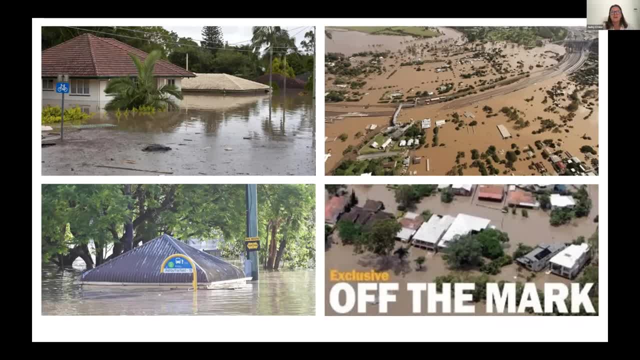 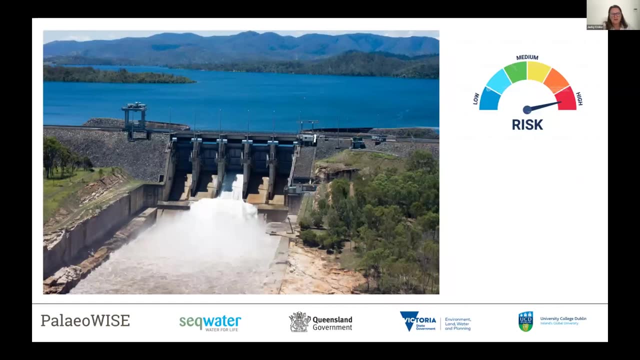 And really what that project was about was actually looking at how we quantified the timing and magnitude of those extreme events. In particular, it was looking at how we quantified the timing and magnitude of those extreme events- And it really Carrick what you said to me there and how we quantified it- the most characteristic of한�one for one or all. have to video, are you just? are you just flowing out the�? you know, in the context of short records here in Australia, The relevance obviously to SEQ Water, who is the largest, you know, Queensland Water Supply Authority, is not just in terms of managing dams, storing is. 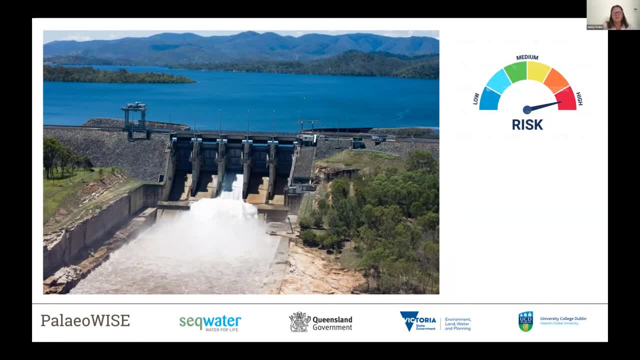 We've heard many tells now of major dams, storages in both Sydney And indeed Wivenhoe here, other places up north overspilling. We're constantly concerned about dams overspill growing population, particularly here in South East Queensland which is one of the fastest. 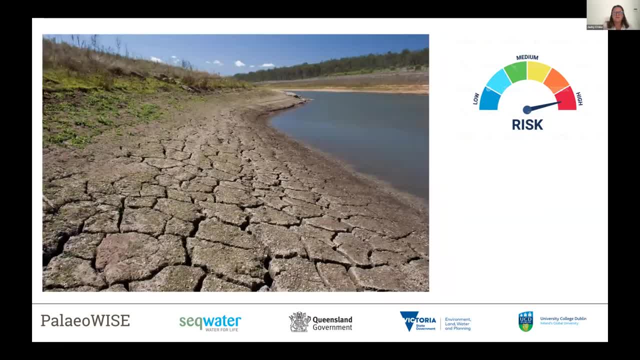 growing areas in Australia at the moment. But the flip side of that relates to the DCAP work, which is around the better prediction of drought events and indeed the management of these. So it's very much that extreme variability of climate that we associate now with Australia which 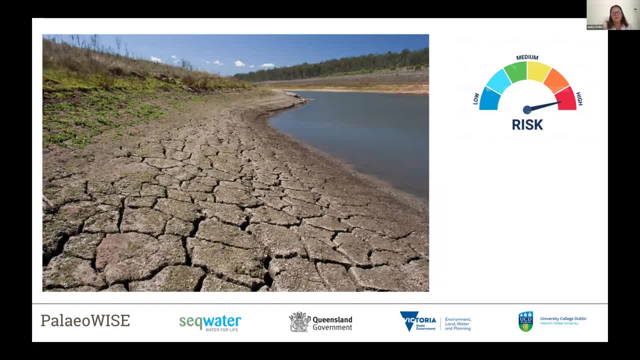 represents the real challenge for people and landholders and stakeholders with respect to water security in general. All of it comes back- and everything I talked about today really comes back to how we quantify that risk. So risk is a function of the likelihood or the probability of 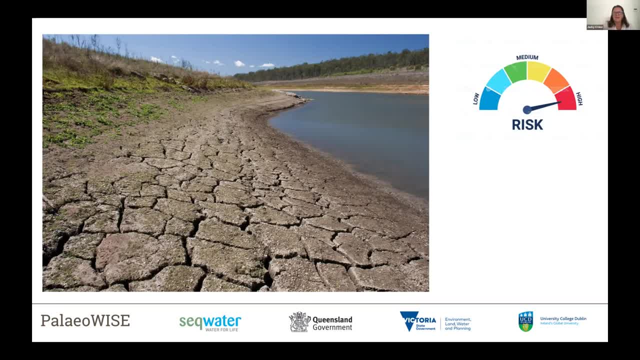 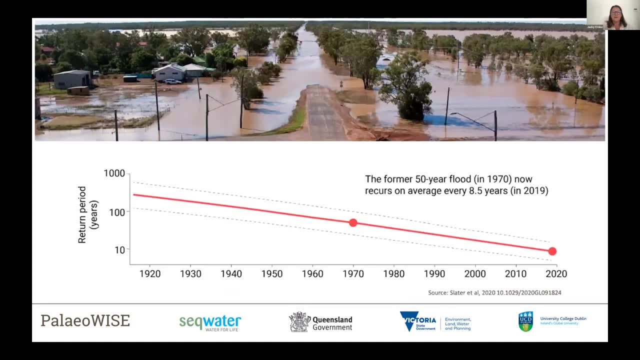 these events occurring and indeed their consequences. So looking at everything I say today within that risk framework is possibly helpful. As a context for this, my colleague Louise Slater from Oxford University published a really interesting article two years ago now actually- I've put the link up there- And she did a global 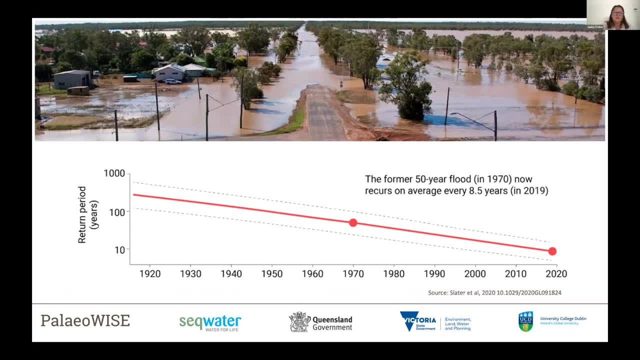 analysis of the changing frequency and duration of rainfall events, And I just thought it was very compelling that really one of the key findings of that work was that you know, the return period of these large extreme rainfall events are actually changing. So for example, if you look at the rate of rainfall in Australia, you can see that the rate of rainfall in Australia is actually changing. So, for example, if you look at the rate of rainfall in Australia, you can see that the rate of rainfall in Australia is actually changing. So, for example, 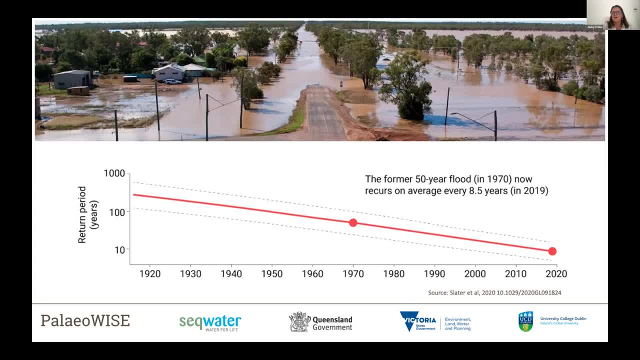 the former 50-year flood in 1970 now happens on average every eight and a half years And I think everybody in Australia has this sense. you know, since 2011,. we experienced another extreme event here in Brisbane in 2013.. We've experienced another one now in 2022, that the frequency 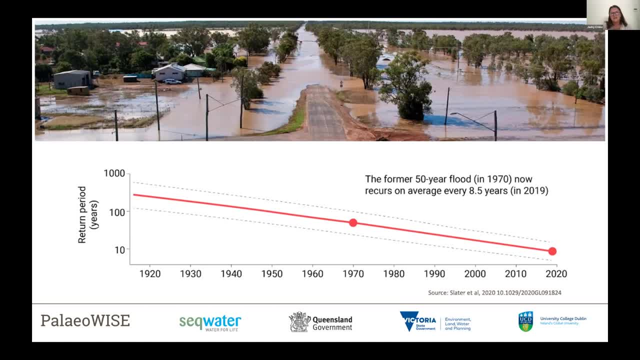 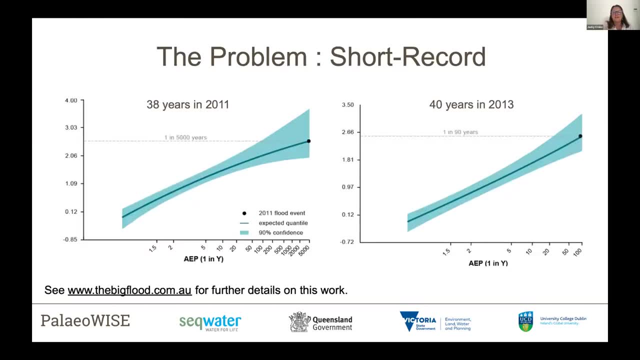 and indeed the magnitude of these events is actually seemingly getting closer and closer. Really, one of the problems that we face here in Australia is the length of our gain and loss of water. So, for example, if you look at the rate of rainfall in Australia, you can see that the rate of rainfall in Australia is actually getting closer and closer, And I think everybody in Australia has this sense, you know, since 2011,. we experienced another extreme event here in Brisbane in 2013.. We've experienced another extreme event. 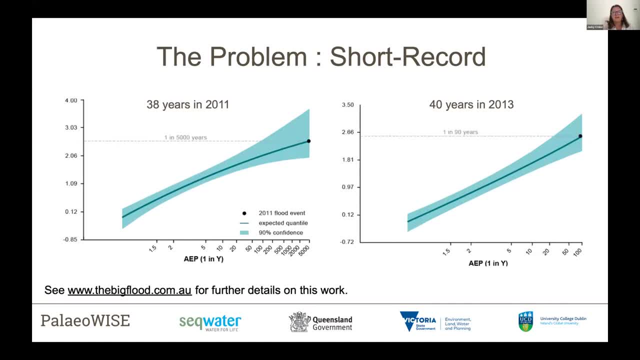 which in many parts, is less than about 100 years. If you're lucky, in many cases it can be as short as 40 years, And one of the most compelling examples that we found of that was actually in 2011,, where we wanted 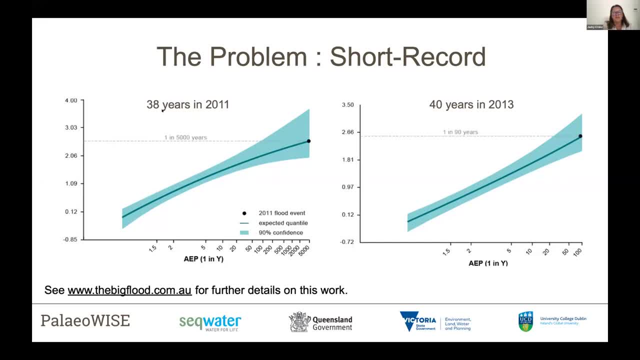 to work out the frequency, the duration, yeah, the return interval for the 2011 events And at the time of that event, using 38 years of data, it worked out to be about a one in 2000.. One in 5000, actually extreme event. Now, two, two years later, when we had another extreme event, 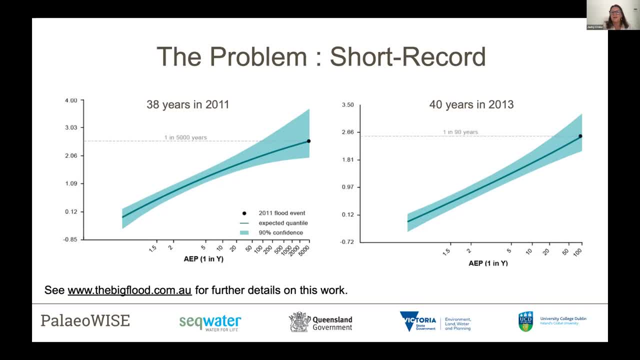 in 2013,. we recalculated that return interval and it had dropped to a one in 90 years. Now that's simply a function of changing both the record length but also, most particularly, the inclusion of these extreme events in the record. So every time we have a longer record, the 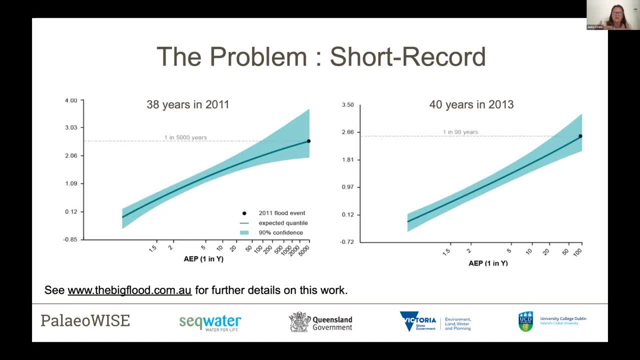 probability of including additional extreme events is going to be lower, And so you know, we're constantly changing that probability or that likelihood And that's compelling in itself. So really recognising that that record is very short and we understand about Australia's climate. 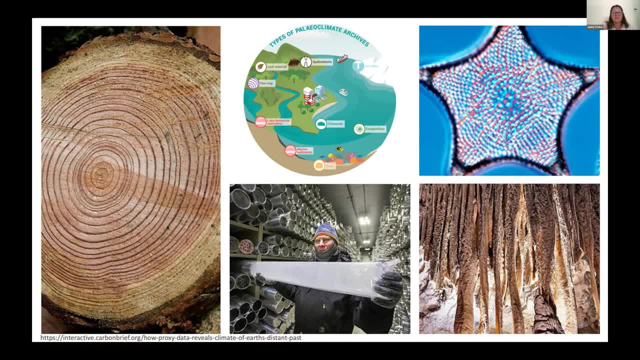 being heavily linked even to decadal changes, such as linked to the IPO and other major climate drivers. The big question was: you know, can we extend the length of that record so that we're capturing a much greater degree of that known variability? 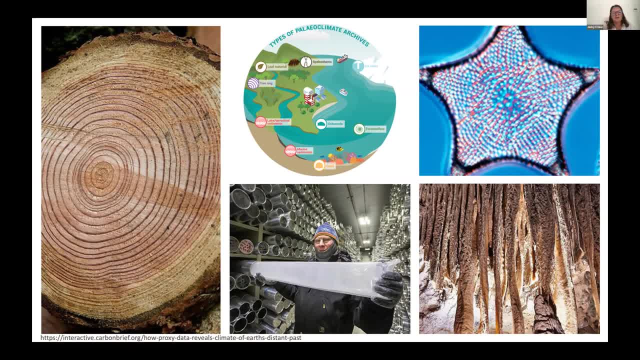 So the answer is that we do have records. we have what's known as proxy climate records, which, which are basically a surrogate for climate often retained in major ecosystems or part of the biosphere. for example, the most familiar one that you might know is tree rings. 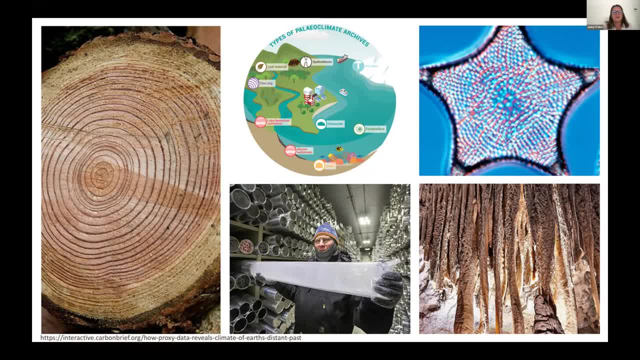 for example, in the Northern Hemisphere, for example, these records are now routinely used to build up a much longer record, say of rainfall in many areas. Other aspects that you might, or proxies that you might, be familiar with is ice cores from Antarctica. 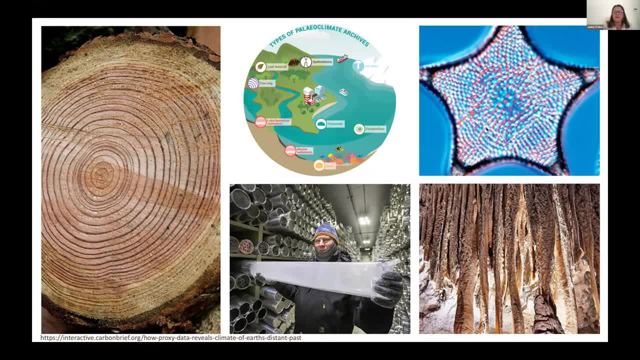 stalagmites, cave deposits, foraminifera and sediment. So there's a whole wealth of this proxy data out there that is compiled in global databases, for example, such as NOAA or Pangea, And the question we started with this project is: you know, wouldn't it be great that the water 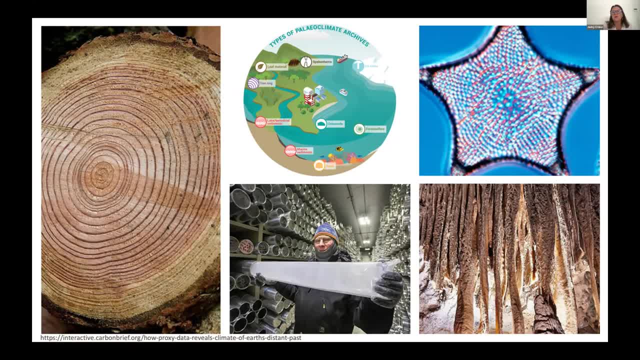 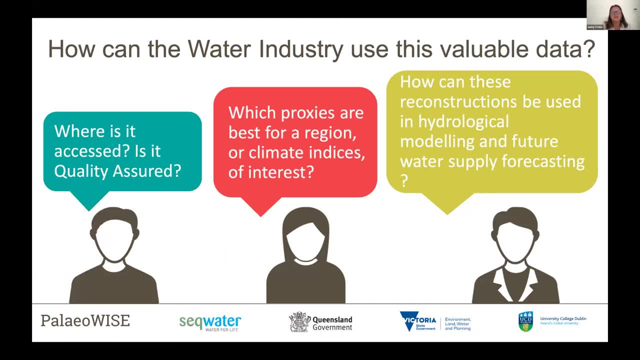 industry had access to this data in a manner that they could actually use it to create a model that they could actually use. So you know, the questions that we started with is: where do they access this? In fact, where is it accessed And is it quality assured? It's not as simple as 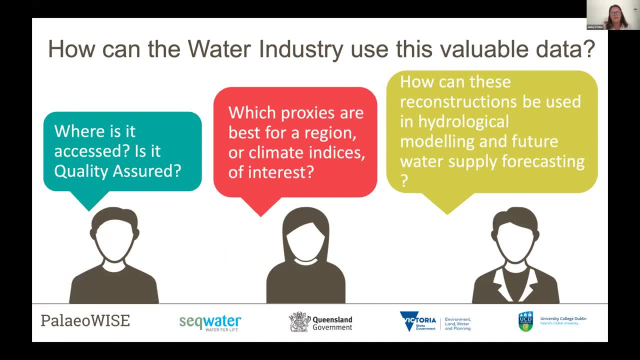 saying to a water industry or a water body authority like SEQ Water, for example: there is this information. where do they get it? You know which of those proxies are best for a particular climate index, And how can they use that information then in hydrological modeling? So those are the 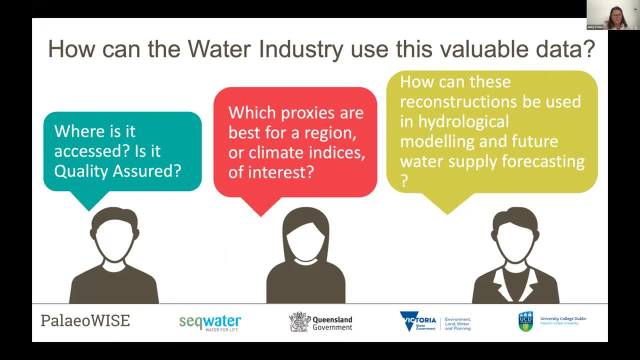 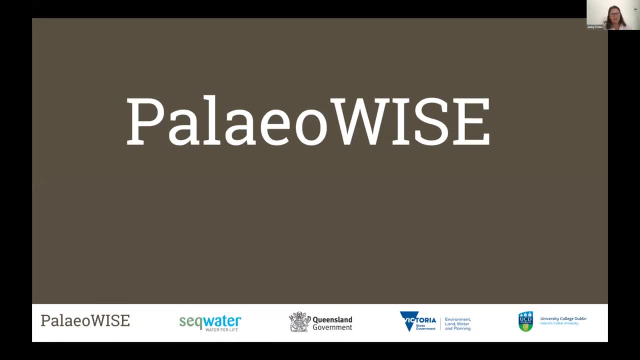 broad three questions that I'm going to try and answer today. With respect to the first one, where is it accessed? Prior to this project, really, there wasn't a standardized database that you could go to that had all the relevant proxy data compiled. 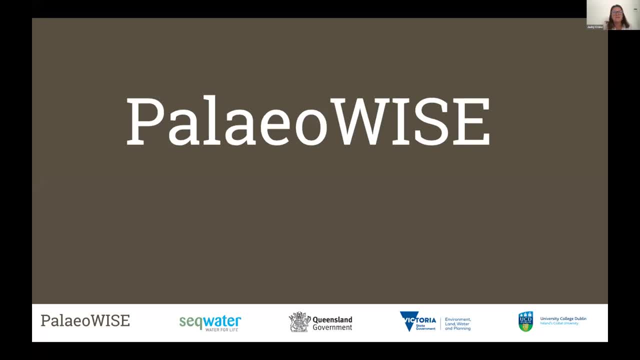 for the Southern Hemisphere. People like Bromma, Dixon and Mandy Front had done fantastic jobs at compiling proxy records- relevant high and low resolution proxy records relevant to parts of Australia, but there really wasn't an open access to the data, So you know there wasn't a. 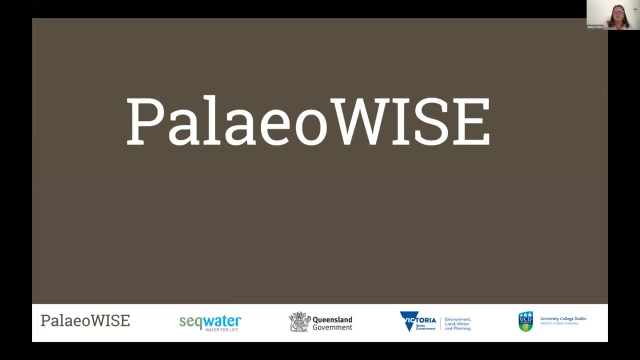 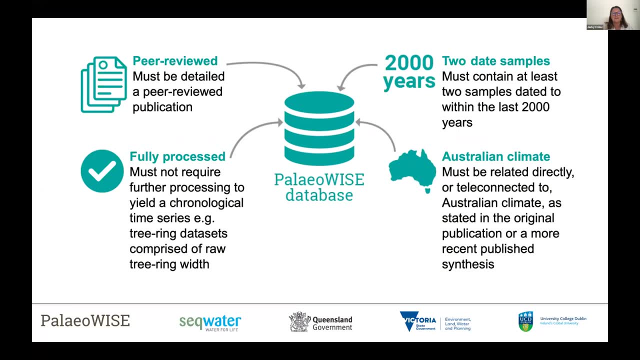 database that people could go have a look at which proxies were available and which ones were most correlated to a particular climate variable. So we set about this. we accessed, you know, hundreds of peer-reviewed articles, for example. We wanted to focus really in on the last 2,000. 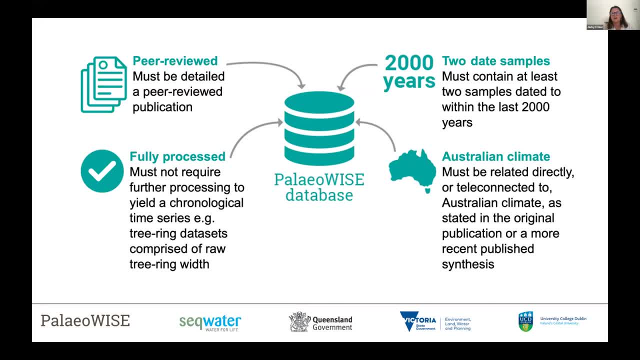 years, The high resolution proxy data sets were our priority. They had to have a link- a pre-existing link- to Australian climates, as previously stated, And they had to have a link to the Southern Hemisphere And they had to be fully processed. So we didn't want to include for. 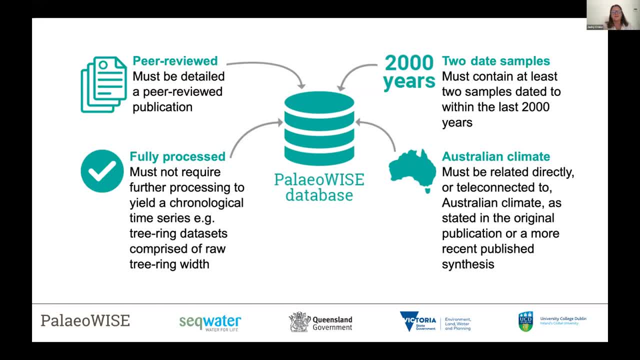 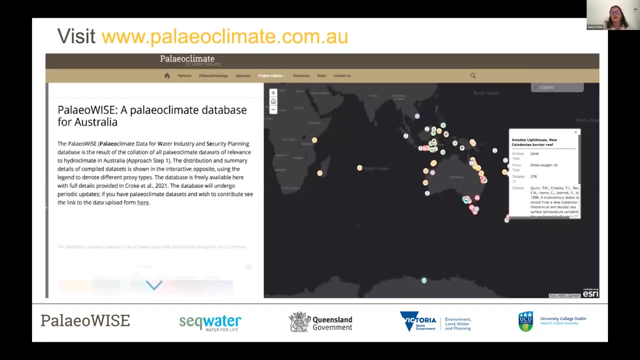 example, tree ring data sets that required us to do any additional work, So they were fully processed, Excuse me. So together we put together what's known now as the PaleoWISE database. It includes 396 records of paleoclimate for the Southern Hemisphere. You can, the easiest way to- 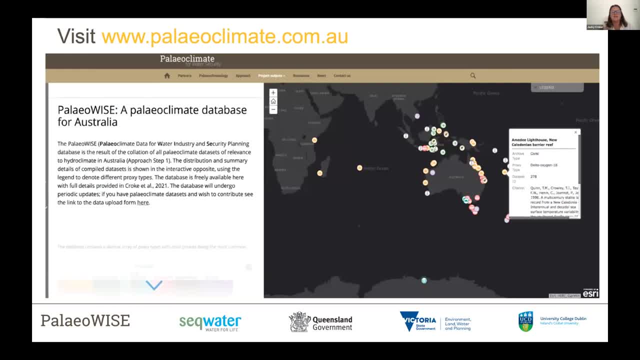 review these, because I'm not going to spend too much time on them today- is to hop onto our website, paleoclimateorg, And you can see that there's a lot of information there, And you can also go to our website, which is listed above there, paleoclimatecom, And you can go in. 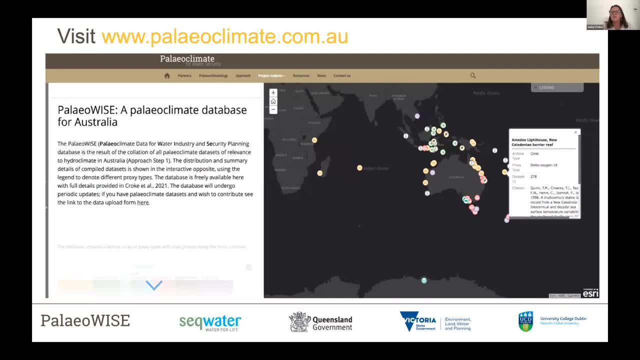 and interrogate each of those proxy records. It provides the link to the original paper, It provides the lat-longs, It provides the resolution and the time span. So that was the first. So that's available on the website. We also wanted to make sure that the database was constructed in a way. 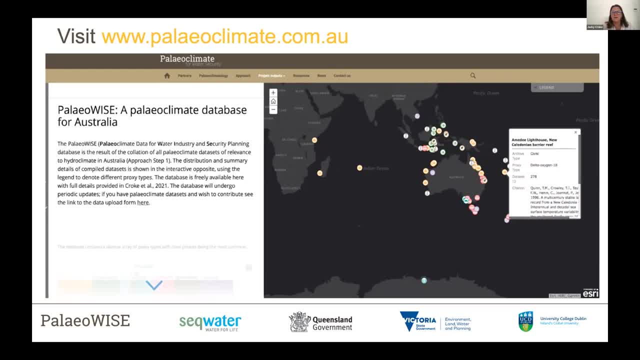 that it was. it could also be searched by other databases. So it's now, with computing power enhancing, for example, it's now getting more and more common, so that we have global databases of temperature, for example. We've got other databases, So we constructed the database in. 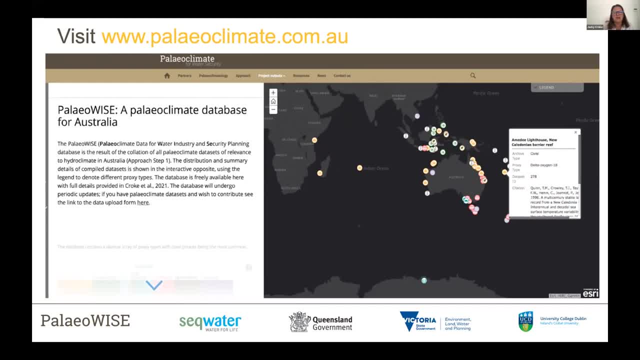 what's known as the lipid format or linked information, paleo data, And that means that we can update it, but also other researchers can also integrate the database into their compilations. All of that data was published at the end of last year in Nature Scientific Data. 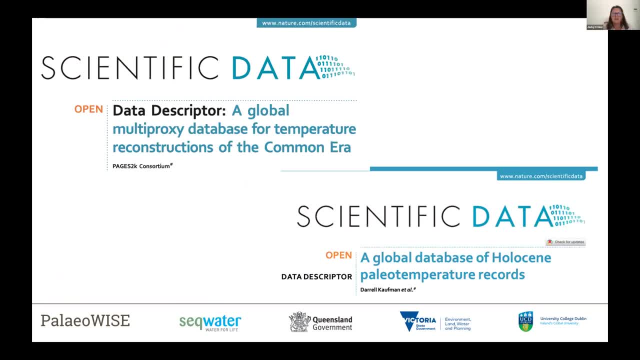 The paper title is up there. If you hop onto our website you will also be able to download that paper directly. So the database is freely available on open access. All of the correlations that I'm going to show you next, the codes to produce those, are also available, And we give some illustrations. 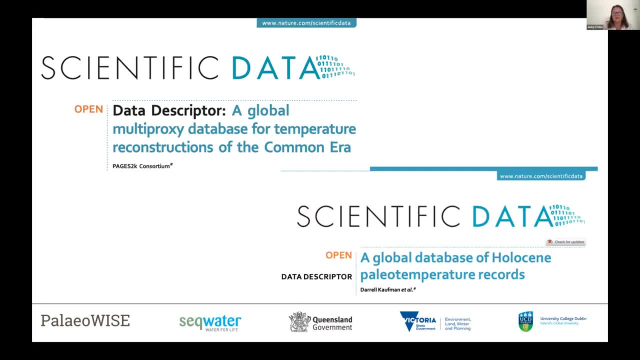 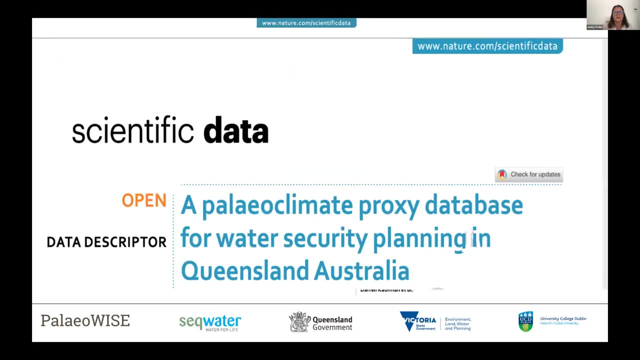 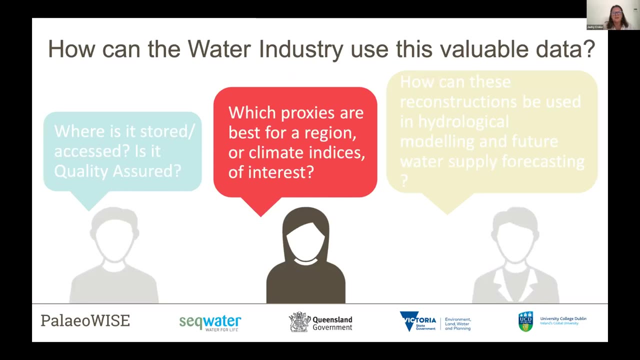 of its, of its application. So we're very happy to see that database published at the end of last year, as it really forms the foundation for the work that I'm going to go on and focus on. So the real question, then, is: that's the record. We have 396 quality assured proxy records there. 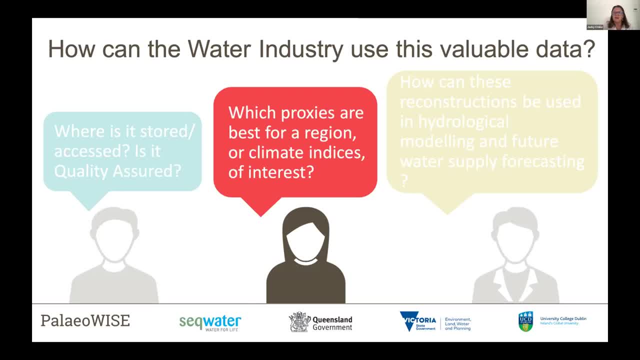 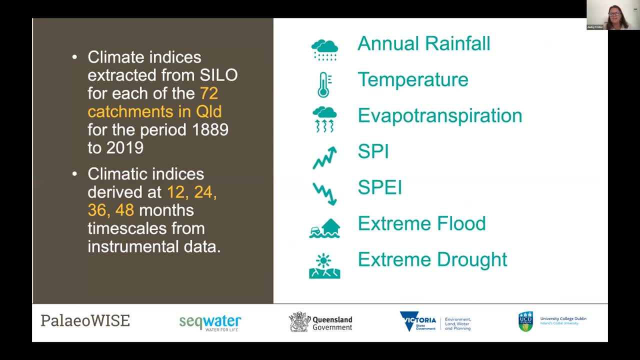 which one of those are best, both for a region or or a climate interest, a climate indice, sea of interest. So what we did was we focused on nine climate indices ranging from rainfall temperature, SPI, which is the standard precipitation index, and SPEI, which is the 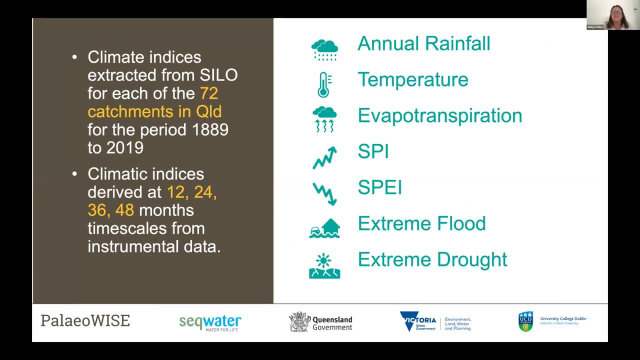 standard precipitation, evapotranspiration index and various indices of Here we go, indices of extreme floods and droughts. So we extracted these using a silo database for each of the 72 catchments in Queensland over that historic period from 1889 to 29.. And we extracted 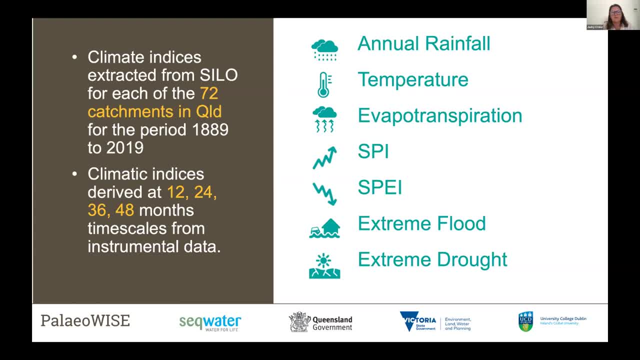 the climate indices at a range of timescales from 12 months to two years and so on, And we did that to be able to look at potential lags in the correlation. but also some proxy records may not respond. You know, if we're interested in SPEI, for example, the more extreme droughts that 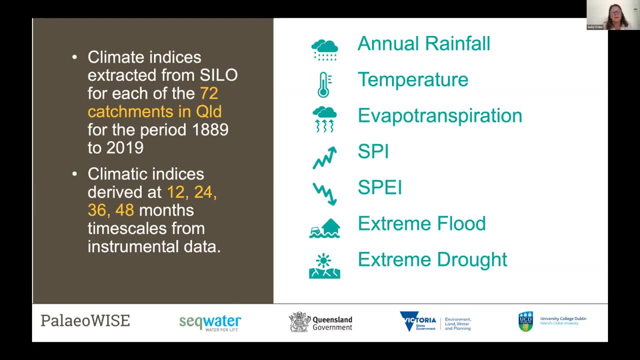 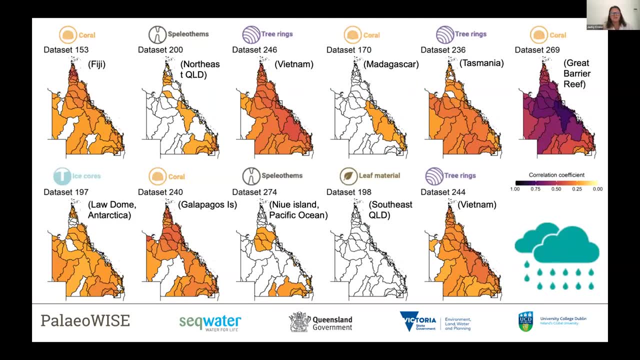 we might be looking at, for example, may not appear for that period, you know, two to three years, for example. So it's quite a compilation. I'm just going to show a couple of results. This again is available in the paper and on our website as well, But this is just a selection. 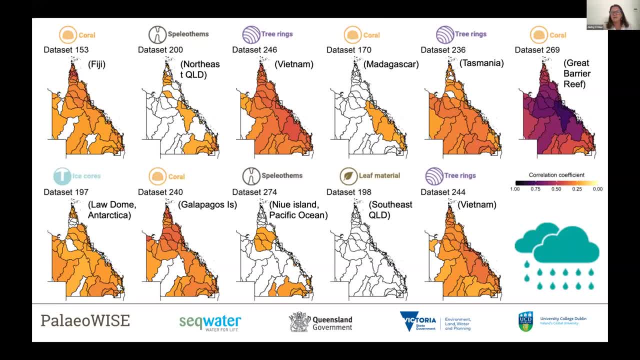 of the correlations between the proxy records and rainfall in this particular case. So the deeper the color there, the higher the correlation. So you can see in the example to the far right of the screen there with the coral example, there's some very high correlations. 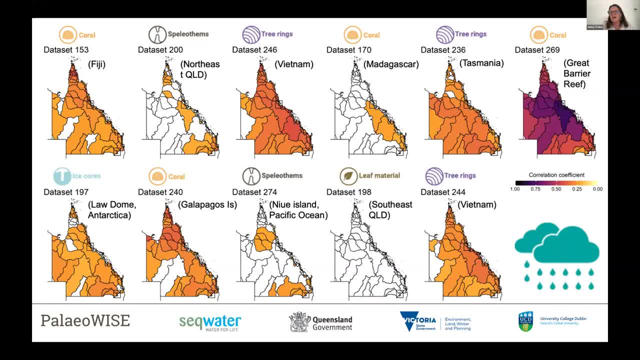 up to about 75% actually between the coral proxy and the annual rainfall for selected catchments in Queensland And you can see the spatial extent demonstrate that that proxy has a large influence really on statewide precipitation rainfall. You can also see that others, for example, such as the speleothems, may have more relevance in selected catchments. 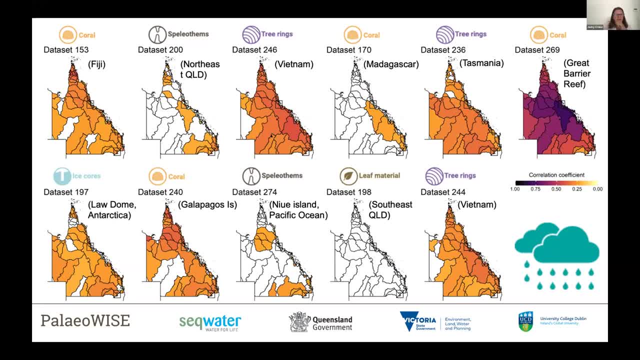 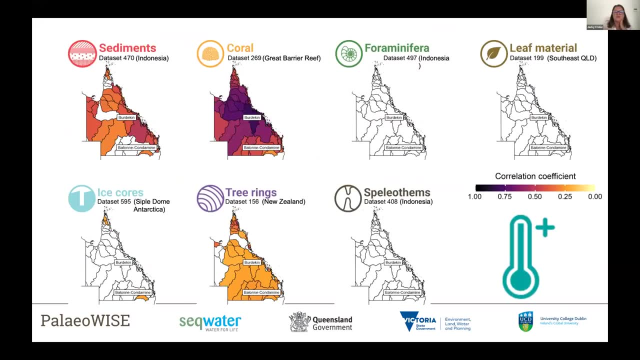 the same thing with the tree rings. So this provided an indication of- excuse me- which proxies had a good association between rainfall in this case, and individual catchments. So this was all done at the catchment scale. This is just a snapshot of the similar output for temperature. 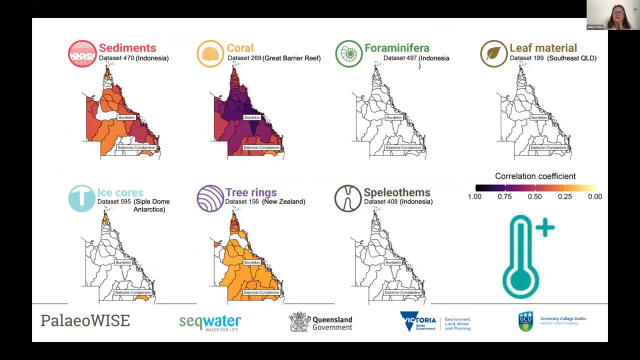 for example, And you can see that corals, yet again, are the dominant proxy record here for producing good correlations, In particular the coral database that Janice Lough was involved with, where coral cores were extracted off the coast of the GBR, the Burdekin and Fitzroy, for example. But you can see the performance of speleothems or foraminifera. 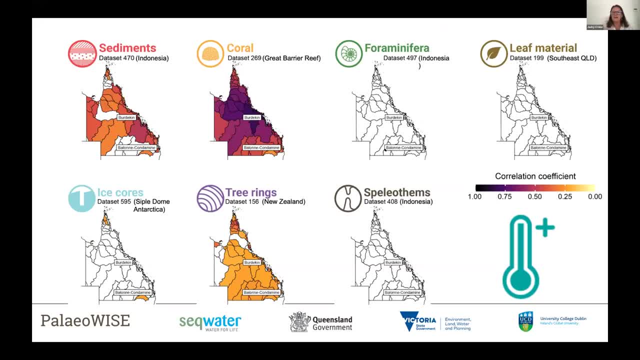 in each of these cases was obviously quite poor. So this analysis allowed us to identify which proxies were useful in the reconstruction of the climate index. you know of interest, whether it was rainfall or temperature. It also allowed us for the first time, I think, to start to see the spatial extent. 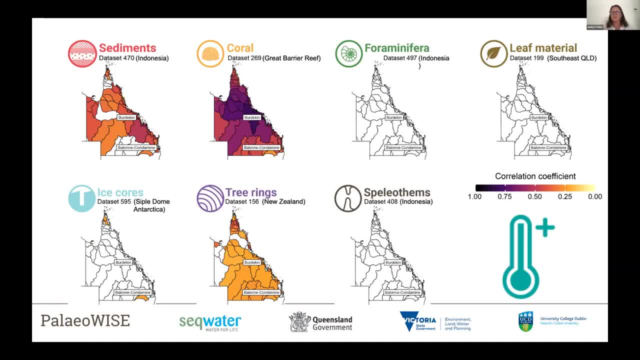 of some of the proxy records. We've never really known to what extent would a coral core from, you know, the Burdekin, for example- apply to other parts. But we can see in that particular instance that there's actually good correlation for a large part of Queensland. 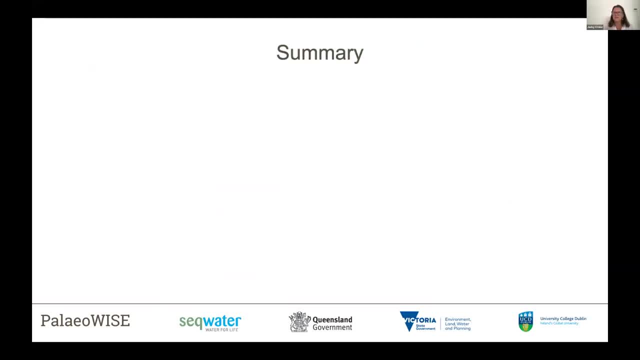 So for the database for paleo-wise, what we did was we put that together into a quality assured data set. All of that is open access and freely available now to everybody. We also had a look at the geographic distribution of those proxies. You know this can be of use to. 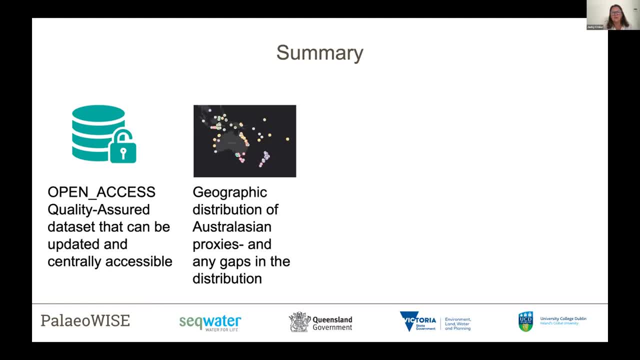 any researchers working in paleo-climate research, for example, because we can start to see the gaps in some of the proxy records available. You know Queensland is relatively fortunate in that we do have a reasonable density of coral records, for example. 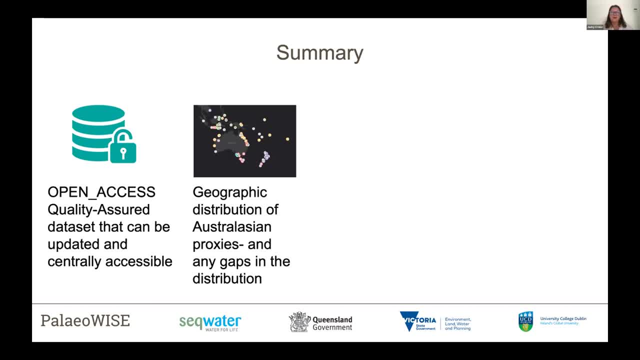 But there are many parts of central Queensland and other parts of Australia, for example, that are relatively poor. It also allowed us to quantify, I think you know, over a large spatial scale which proxies were best for a given climate variable, And they weren't necessarily. 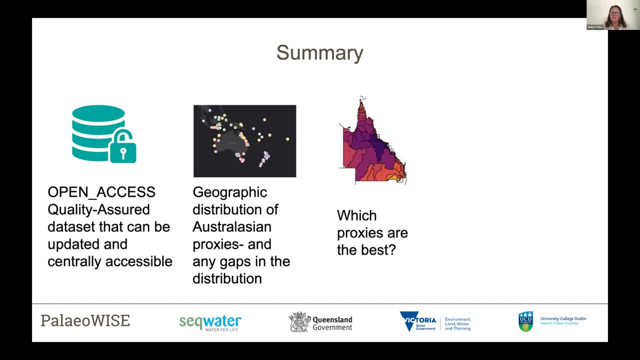 the same. In general, the corals perform best for rainfall and variables like SP DEI. other climate indices were also better aligned to tree rings. So corals and tree rings, I think, provided the majority of our correlations. So that was what we produced in that. 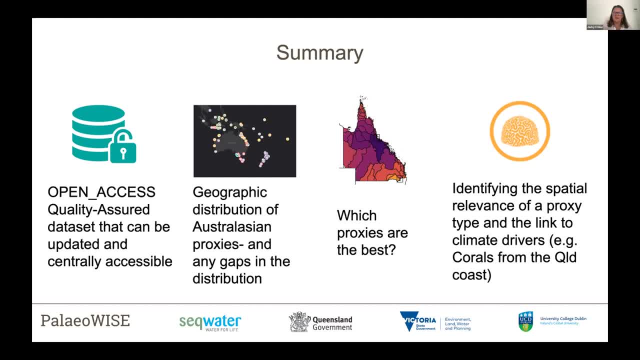 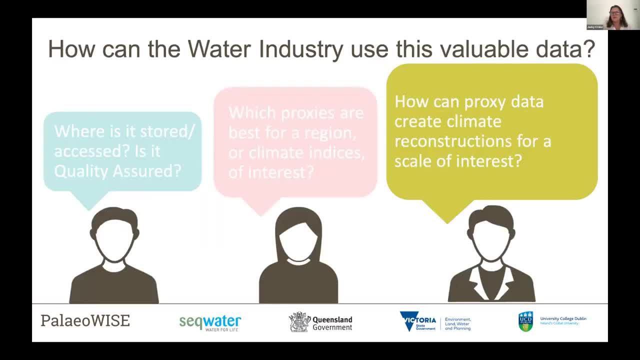 phase of the work which was a large part of the first DCAP-funded project, really, which was the production of that work. The more critical aspect I guess right now is how can this information be used, And in order to do that, we want to be able to do a lot of work on the. 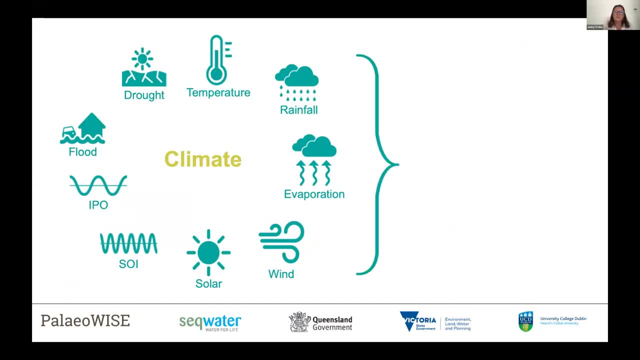 ground, So we wanted to have a look at how those climate indices that we selected- you know, everything from rainfall through to temperature and SP DEI, in addition to some of the other major climate drivers that we're familiar with- IPO, Southern Oscillation Index, and you know 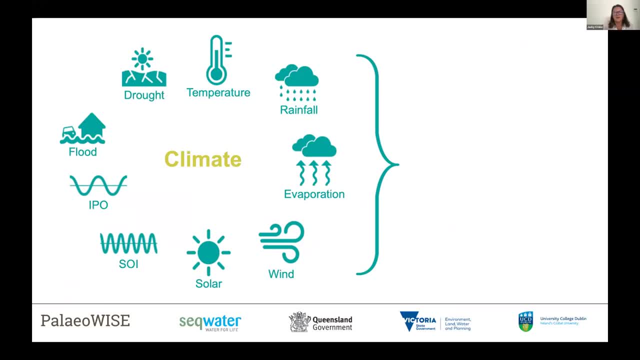 other climate drivers that we know have an influence on. you know that variability in Australia And what we really wanted to do was to be able to extract these at a at a level, a time series level, that we could start to characterize it, that we could start to 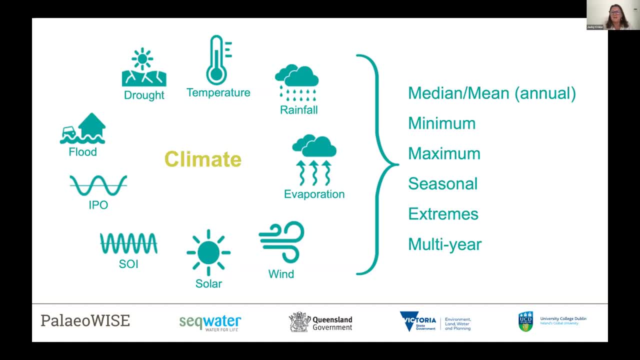 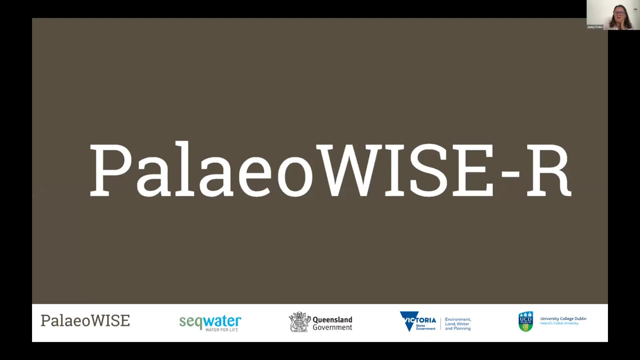 see, you know minimum and maximum variability. We could start to see if there are any seasonal trends and, in particular, that we could start to identify extreme events or multi-year droughts and so on. So this was the second phase of our work, which leads us into PaleoWise R. So PaleoWise. 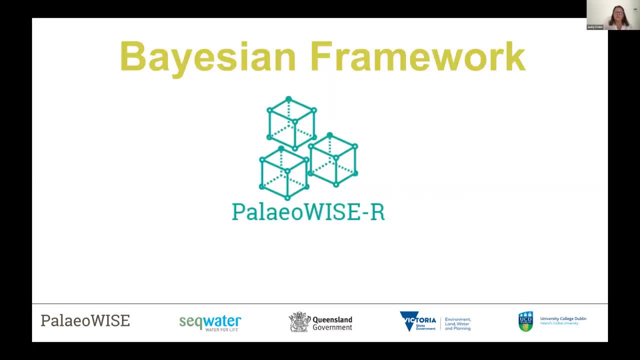 was the database. PaleoWise R is the reconstructions as a result of that. So for this work, which was really done with my colleagues back in Dublin, Niamh Cahill and Andrew Parnell, who are excellent Bayesian statistical modelers, 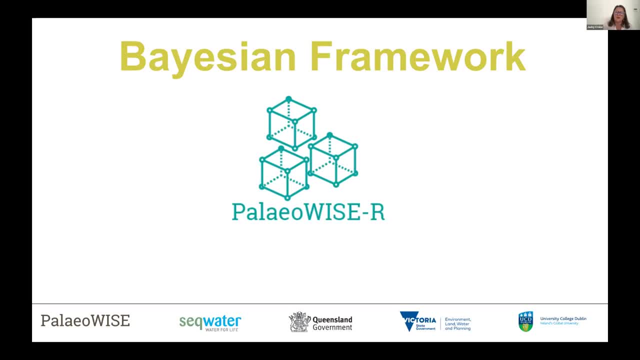 we started having a conversation around this and collaboratively we developed a Bayesian framework. So for those of you not familiar with Bayesian, there's some information coming on our website but effectively it allows you to use all available information. So previous work in this. 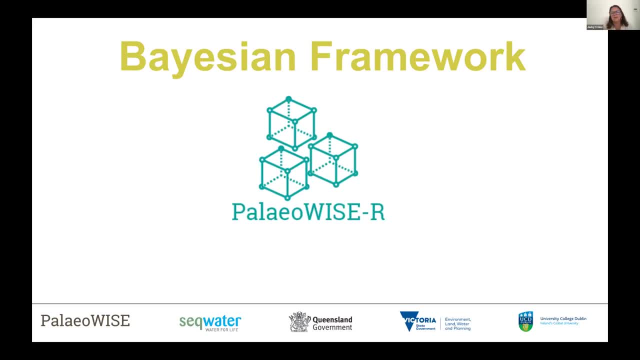 space may have looked at a single proxy, for example, and its relationship to a given climate variable. What we wanted to say is that, well, we can see that there are good correlations between maybe 10, 15 proxy records here spread across that southern hemisphere. How can we actually mine? 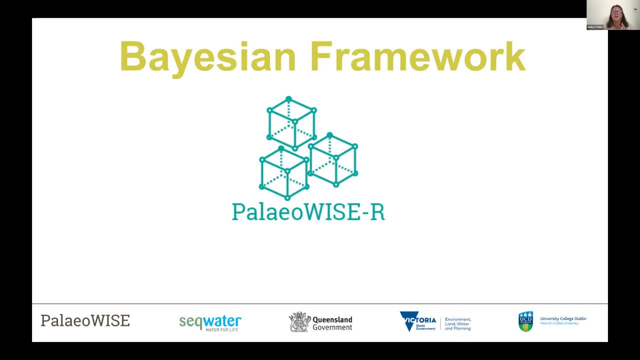 that information and how can we develop a framework that builds in the uncertainty, both in the proxy records and in the model predictions, right from the start? So the Bayesian framework allows you to do that. It's very applicable to a large area, for example. It's as I said, it can use information. 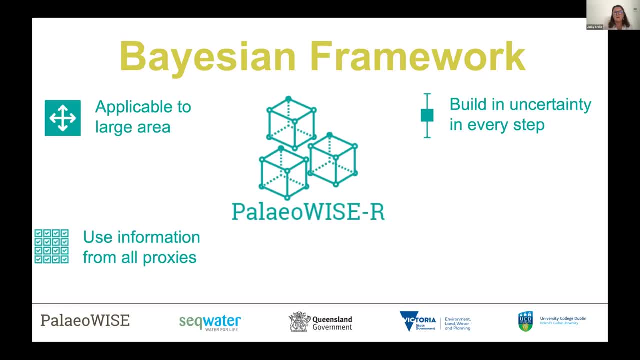 from all proxies and, most importantly for our perspective, it can build in uncertainty. So one of the issues that we face in making predictions, both in terms of past and future climate change, is what's known as the uncertainty around those, and having something that quantifies 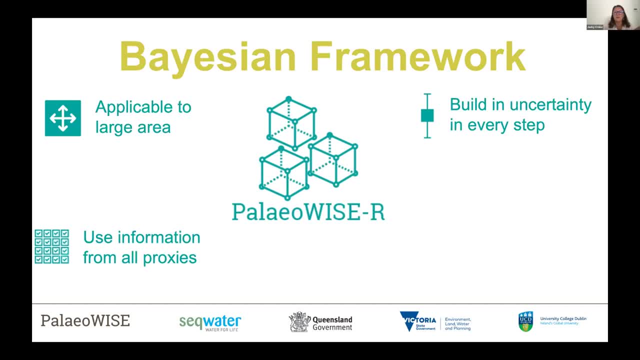 you know, 95% confidence intervals really gives the water security industry that greater assurance. that you know, these are the bands that are particularly relevant, that in order to best manage the you know the timing and the magnitude of some of these events- we really 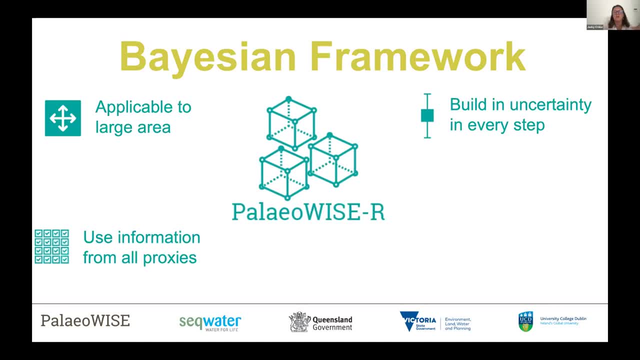 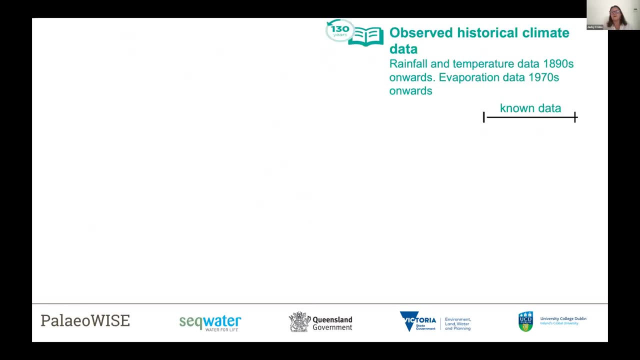 should be looking at within that uncertainty and not just focusing on means. for example, And now that we have access to supercomputing, it's a particularly efficient way of generating reconstructions from a large database. So we did that just very briefly. This paper is now. 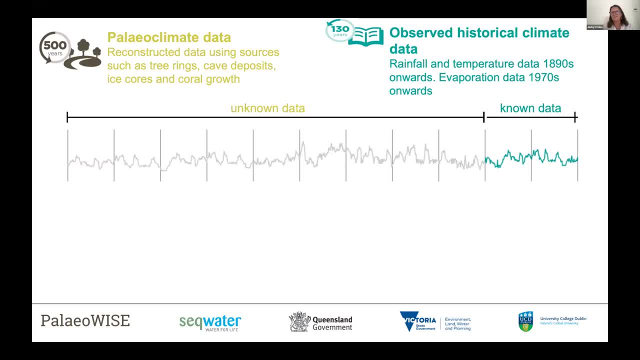 in press and there will be a link there is. you know, there will be a link in our, on our website again, so I'm not going to spend too much time on it because it can get a bit deep, but effectively. 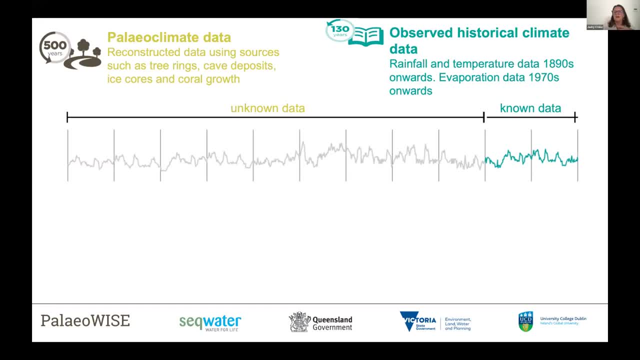 what we have is that historical record which we, that's our observed historical data, which obviously forms a foundation of some of that variability. We had to characterize the time series distribution for each of those climate variables in each of the, each of the catchments. 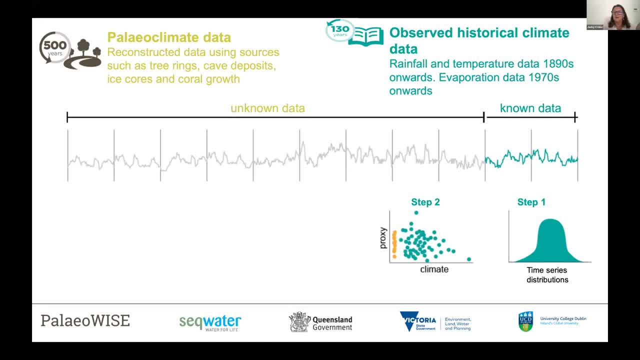 of interest. We then wanted to compare the relationship between that proxy and that climate. There has to be a reasonable representation of the proxy climate within that distribution. If there isn't, the model has nothing to constrain itself, so it doesn't. 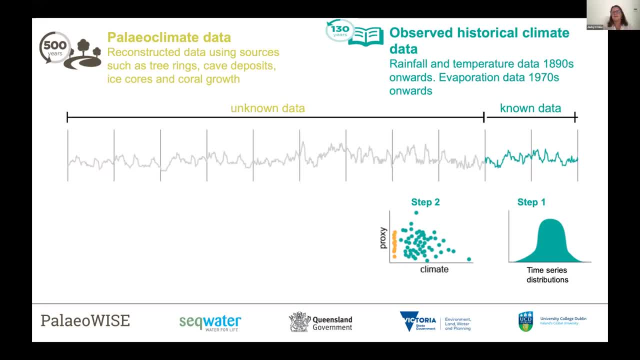 what's known as a convergent test. it doesn't pass a convergence test, and then it's not actually used in the model. Step three, then, is to basically characterize the distribution of both the proxy and the climate, with that uncertainty, and there's a whole process where we extract certain numbers. 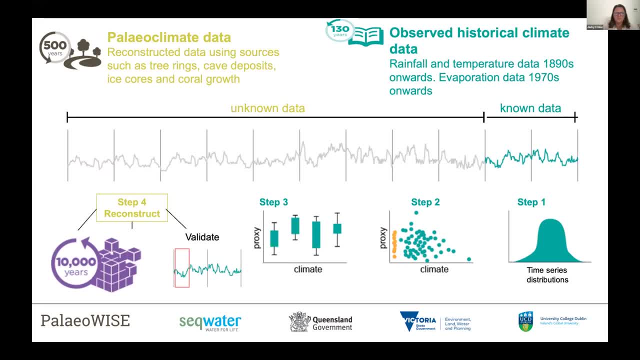 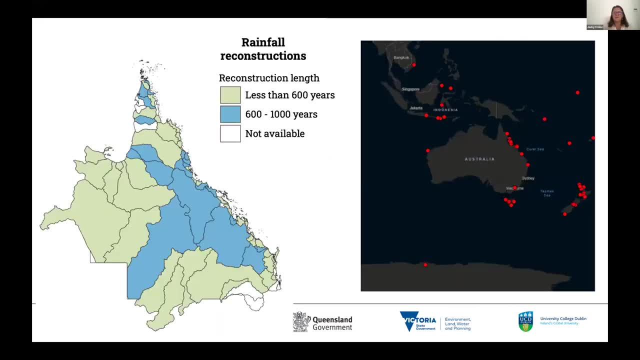 of the data set, the time series to validate and the final step is obviously the time series reconstruction. So that's roughly what it involves. What we found was using output that was maximized for accuracy. for model accuracy, we found that the majority of catchments in Queensland 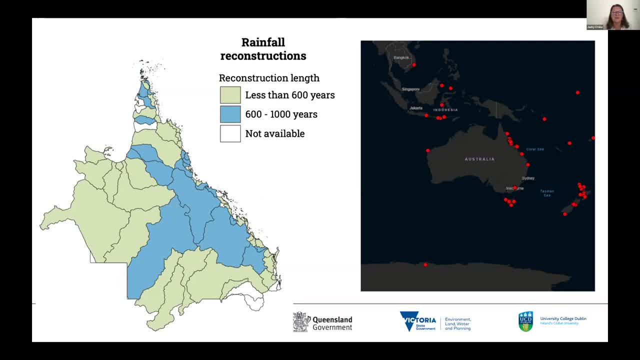 produced a reconstruction. so that is, they passed that convergence test and a reconstruction was possible. Two time steps were evident. One was approximately around 400 or less than 600 years. Other longer time series were up to about a thousand, a thousand years, and you can see the distribution. 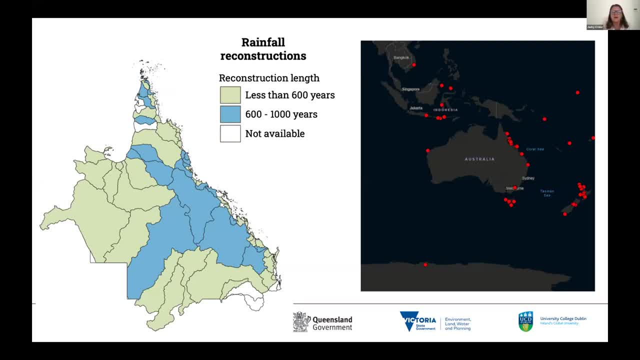 in terms of catchments there. One of the things with the coral records, because they're high resolution, they're annual or less in some cases. the time series of the coral records is about 400 years itself. If it's longer, that resolution tends to drop off. 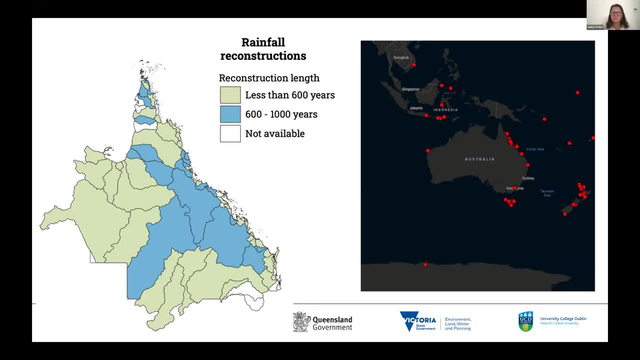 So obviously we've identified that corals played a key role in the correlation with some of the climate variables, so that time scale is somewhat constrained by the proxies itself. In other cases, the proxy records may be longer and have higher resolutions. Now you can optimize the model. 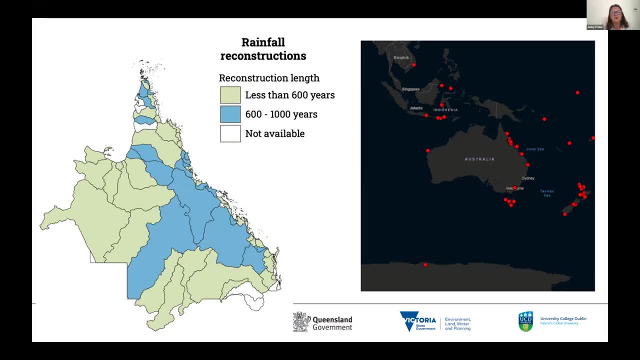 not just for accuracy. If you're interested in a longer time series, you can optimize it for that. but, as I said, we've optimized here for model accuracy. so that's the best available time series, the most accurate time series. So that's the best available time series, the most accurate. 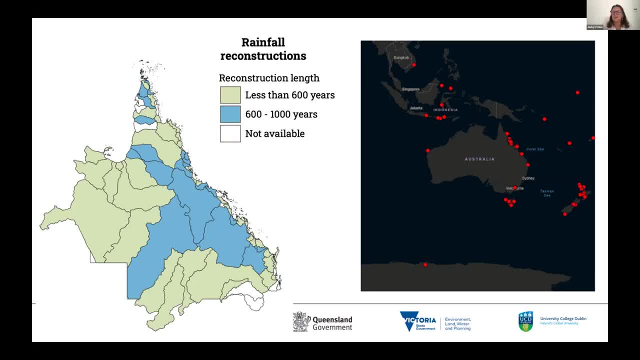 available one. The image to the right just shows you the proxy records that were involved in the Queensland reconstructions and I've already mentioned the coral records close to the GBI there. but as we extend it out we can start to see the tree ring records both from Tasmania and 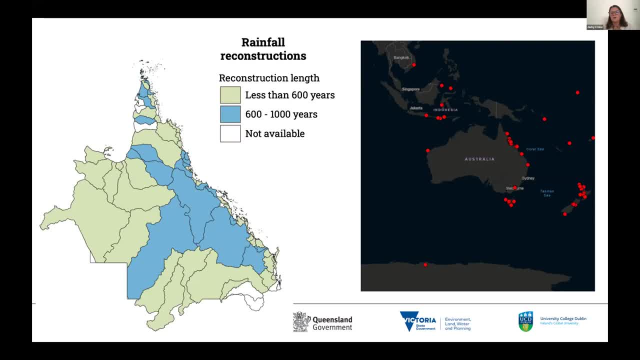 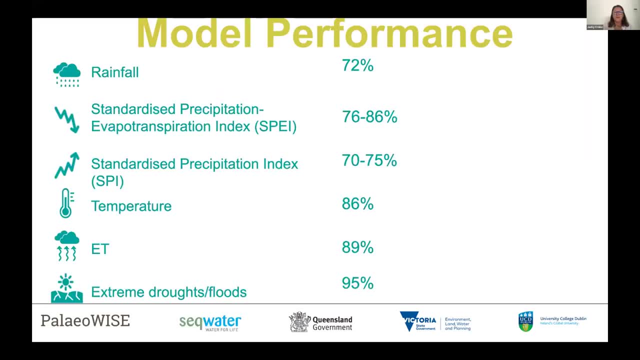 New Zealand and some of the coral and also sediment cores from Indonesia were also coming into our reconstructions there In terms of model performance. so each time you have a reconstruction, for example, it produces some sort of model performance which we've expressed here as a percentage. We'd like that, obviously, to be within that 95%. 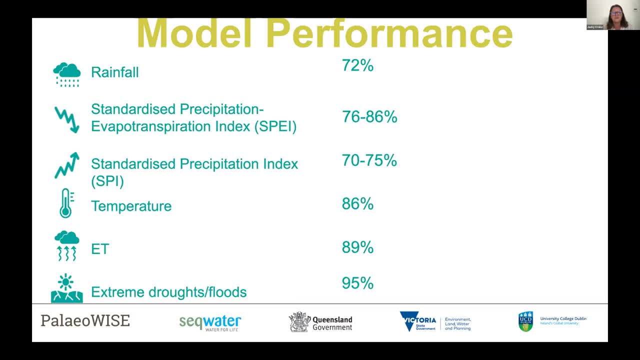 confidence interval and the reconstructions for extreme droughts and floods produce that Overall, the models, across all climate variables, had a performance of about 79%, which means that the model is accurately predicting it about 79% of the total. So some of them were more accurate than others. As I said, you can optimize for model performance. 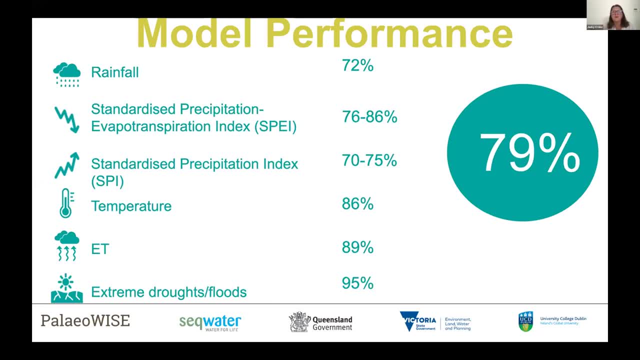 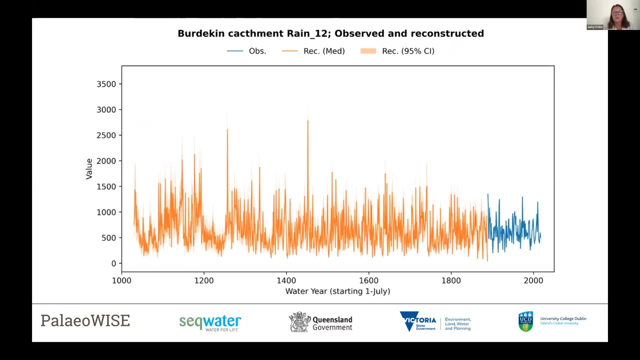 as we've done here, and get a shorter record, or you can optimize for model length and you can determine to what extent that reduction in error actually impacts the application that you're using. So there's going to be a few of these. These are the actual time series reconstructions. 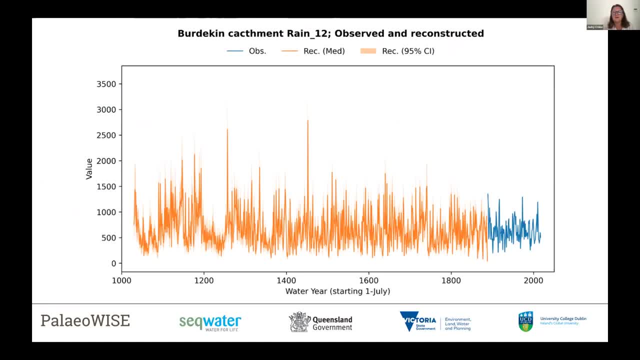 So the primary output from PaleoWise are our time series reconstructions. The blue at the start there represents the historical data and the orange lines represent the annual rainfall reconstruction. This here is for the Burdekin catchment over that 1,000 years. It may be difficult to see, but you can also see the 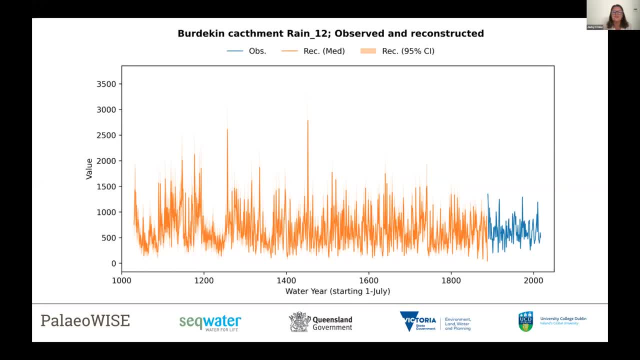 standard errors, the standard confidence intervals there, 95% represented. So even looking at this as a primary data output, we can see that the degree of variability as represented in our historical time period is certainly not fully represented by that longer time series. So we can see considerable higher rainfall values. 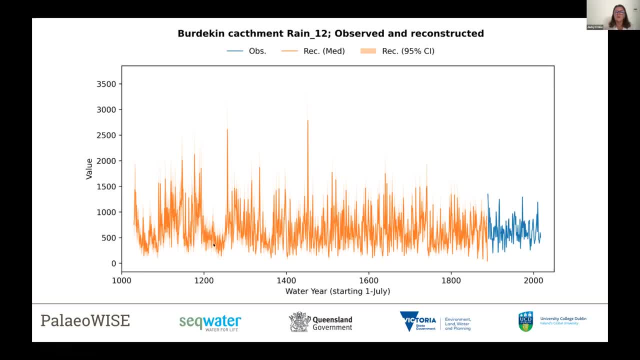 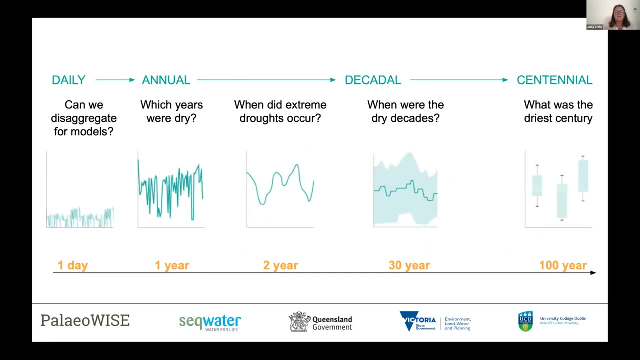 here in that 1,300. We can also see considerably lower values represented than that historic period. To us, the time series in itself is tremendously useful. Most of the water industry would say, well, OK, what are we going to do with that? So what we wanted to display is: 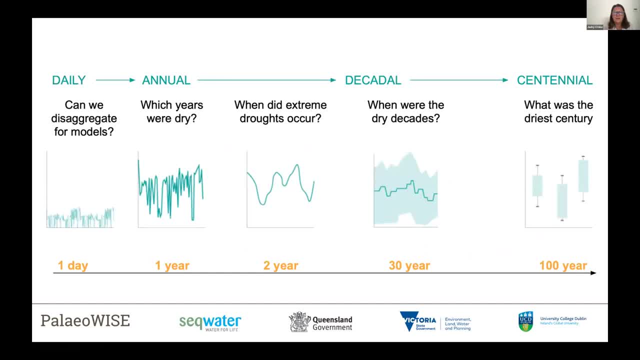 that really, once you have that time series, you can start to look at it in any particular resolution that you wanted. So, looking at it in terms of a daily, you could disaggregate that into a daily time step for some of the water resource modeling. that's been done and I'll 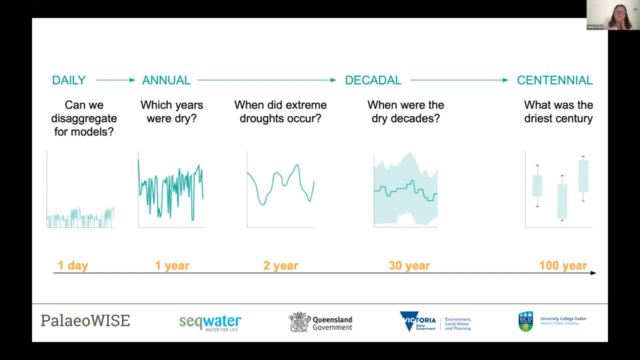 give you an example of that. But you can also start to look at it in terms of annual resolution. which years were dry? When did extreme droughts occur? When were the dry decades? You can start to look at it in terms of estimating statistically. 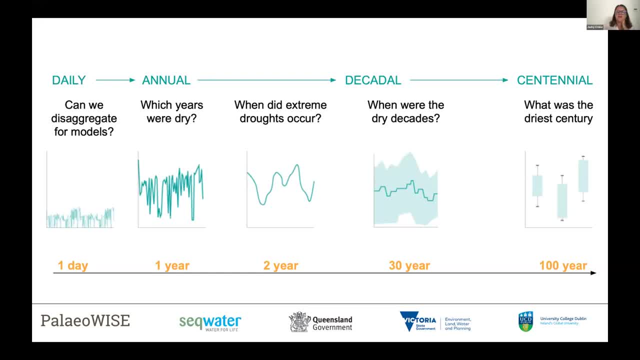 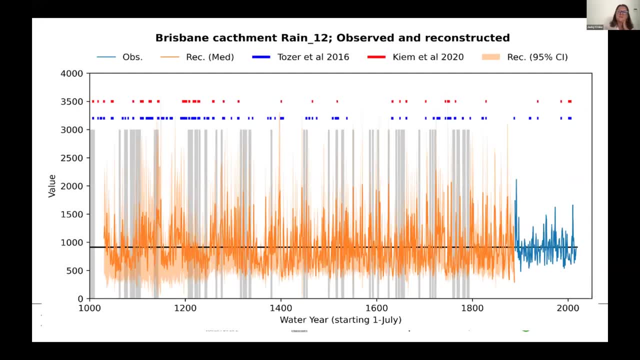 significant change points over that century time scale. So once you have that time series, to a certain extent anything is possible. This is an example here of the Brisbane catchments. This is a 1,000-year reconstruction of rainfall for the Brisbane. Again, the blue denoting the. 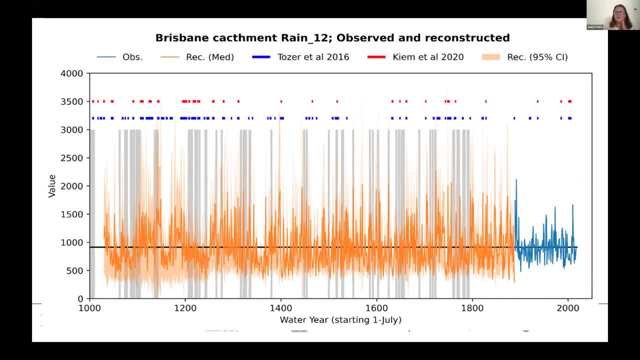 historical period there And we've superimposed on that these gray bars here, which are effectively a drought classification, which was annual, was less than the mean times, the standard deviation over four consecutive years. So these represent dry periods over four years or greater. 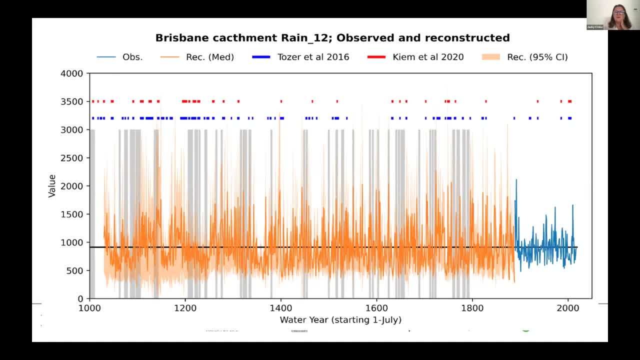 And you can start to see the distribution. The red and the blue dots there, which make the graph a bit busy, are really previous work, Anthony Keams and Tozer's work, which have also identified droughts here in Southeast Queensland. So there's some broad alignment. but 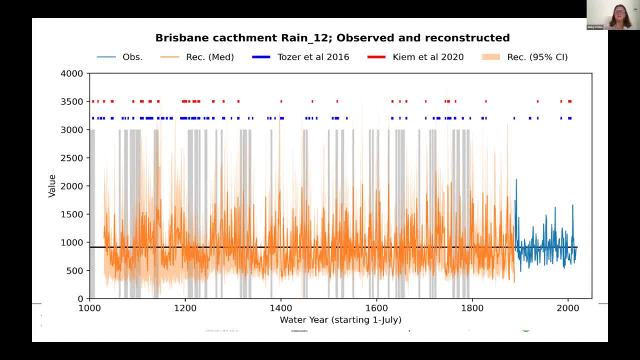 the main point of this slide is really just to demonstrate that once you have that time series, you can apply a series of- whether it's drought classifications or rainfall anomalies. anything is possible. This is just a similar example, really, here, of using 100-year means. 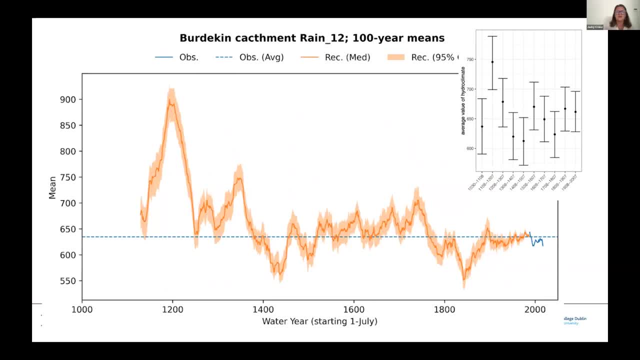 to represent the 1,000-year reconstruction we have for the Burdekin catchment. So looking at it over that longer time scale you can clearly see again with our historical period here what that is. But we can start to see some of that variability, particularly here, in that. 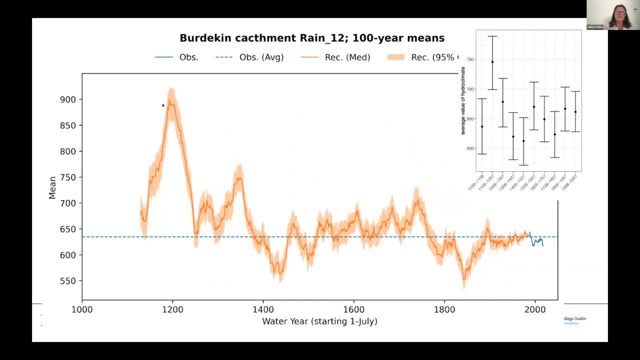 early 1800s. But obviously the big outlier here is the rainfall values throughout that sort of 1,100- to 1,200-year time period. So the inset up here is really just some change detection work that we did, using the values and their confidence intervals to identify which. 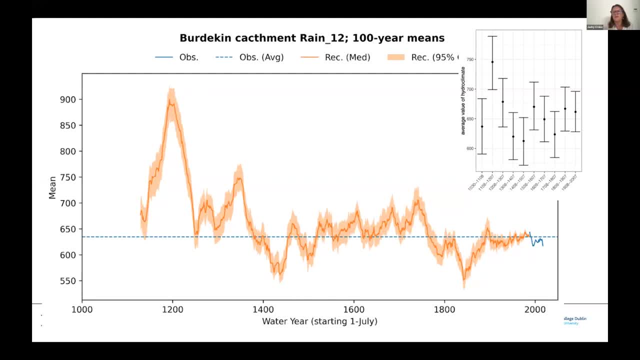 were the most significant changes in those centuries, for example, are significantly different to any others, And you can see that that 1,100- to 1,200-year period there is very significantly different to anything that we've had in any time since, and certainly relative to. 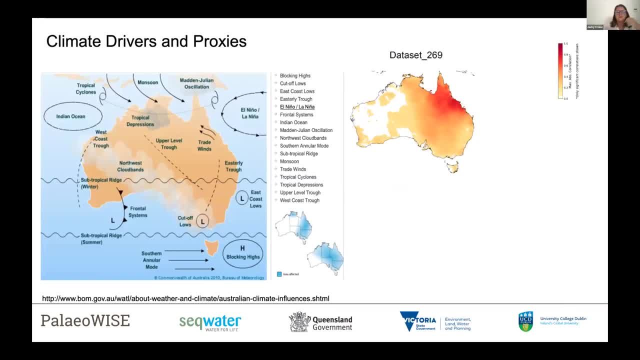 the historic period. What we were also interested in doing was using the database to reconstruct some of the known climate drivers. I've mentioned some of them previously. These are represented here on the Bureau's. We have the climate influences- east coast lows. We have the El Niño-La Niño, the Indian Ocean. 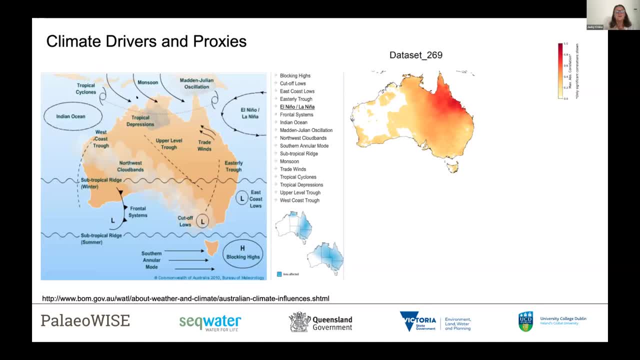 We have the IPO and the influence of the monsoon And from our early work there with the coral work that I showed you the high correlation with annual rainfall, we could see that there was some potential here to use the database to also look at which one of these proxies may be most. 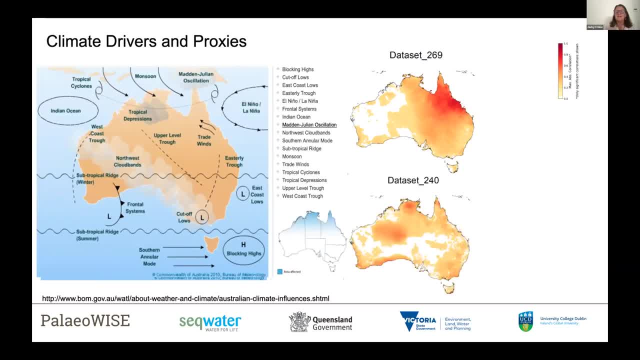 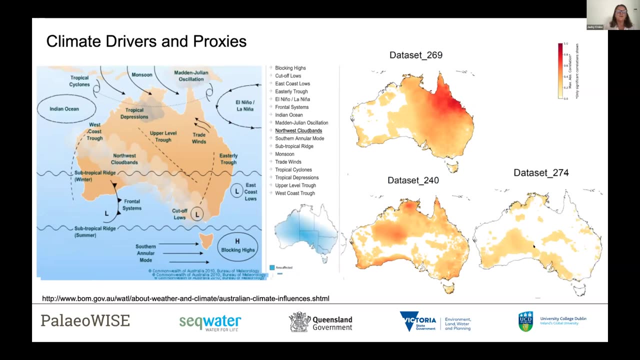 relevant to a particular climate driver. So we can start to see the relevance potentially here of some of the more tropical influences. whereas this one might be the El Niño-La Niño influences that we're seeing in the corals, We can also see others that may be more representative. 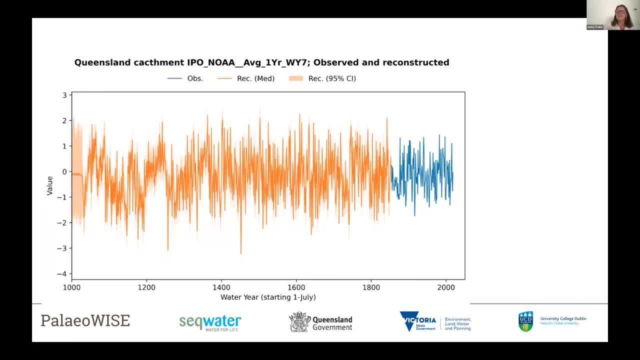 here of the, you know, the Northwest cloud bands and so on. To that end, we use the database to actually also reconstruct the 1,000-year time series for each of those climate drivers now. So this is the IPO: 1,000-year reconstruction Again. 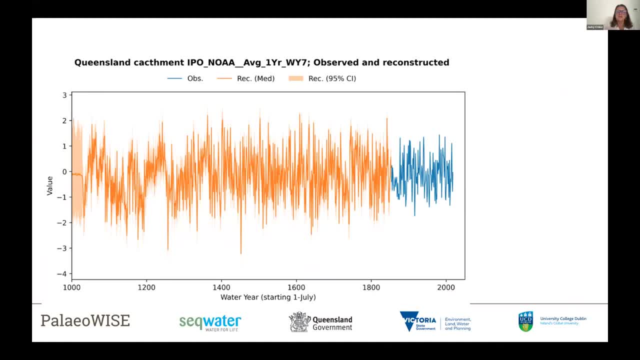 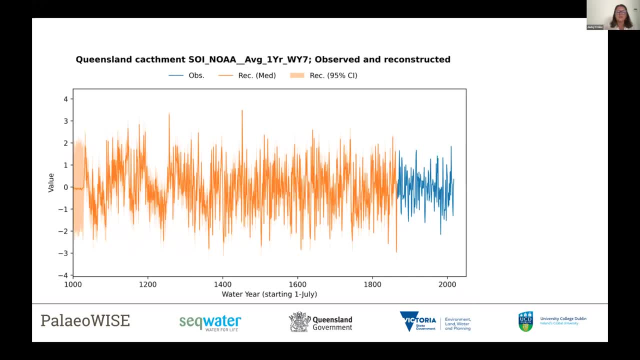 the documented one there in blue, and our own reconstruction in orange, there with uncertainty. And we did this for SOI. I'm not going to show it, but we also did this for IOD, NN34, and so on. So we have now a 1,000-year time series for each of those major climate drivers. 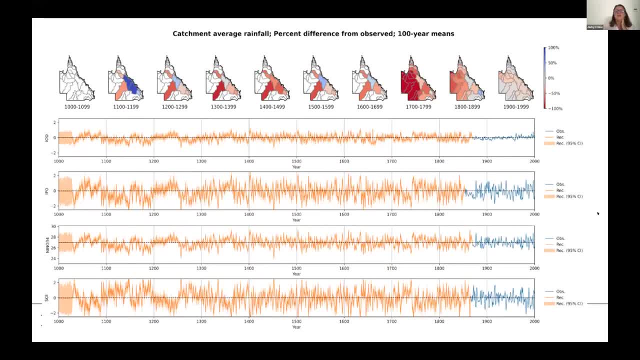 So our intention is. sorry this is a very busy slide, but we're working on a way to actually show the top sequence there. It shows you the percentage difference of annual rainfall relative to the present, for example. So anything that appears very red was considerably wetter, you know, maybe 50, 75 percent. 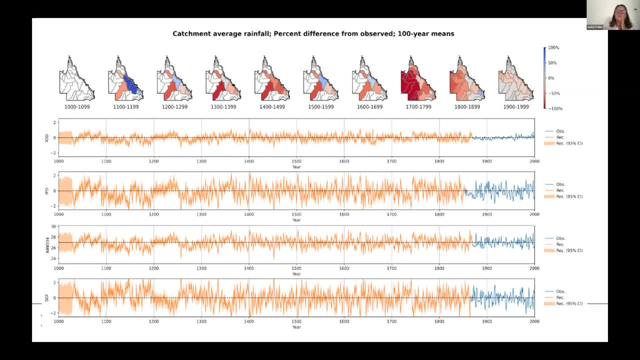 wetter than the historical period. We can see the performance of individual catchments throughout that. Underneath here are the time series for the climate indices, and we're working on this at the moment for a graphic where we attribute each of the changes in 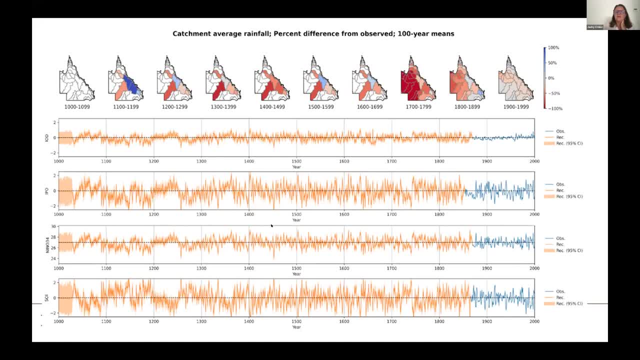 rainfall or SPEI to a dominant climate driver. So in some cases that might be IPO, In other cases it might be IOD and so on. So when this work is finished, we'll have not just a visualization of the percentage changes in rainfall relative to that historical period, but which of those climate. 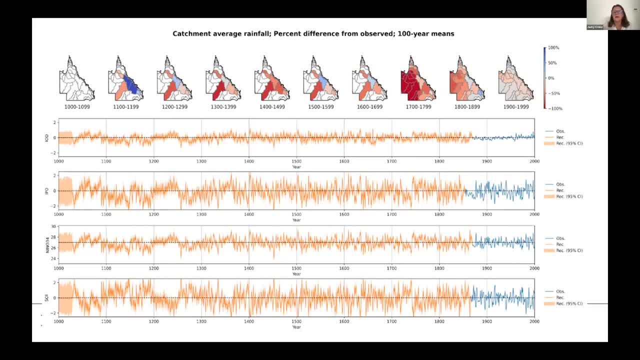 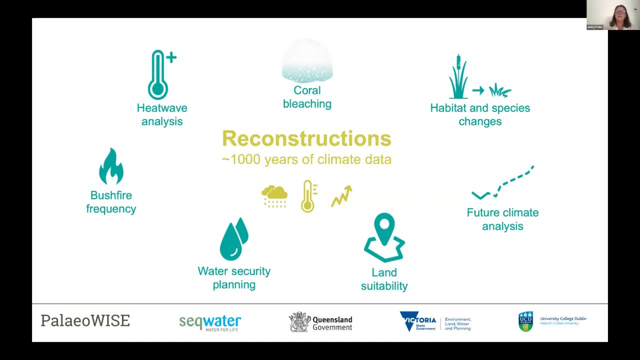 drivers appears to have been the dominant attribution. So that was a very quick overview. I'm hoping I leave enough time for questions. but effectively those time series can be used in you know any number of ways really, And we're very keen that people appreciate that It can be. 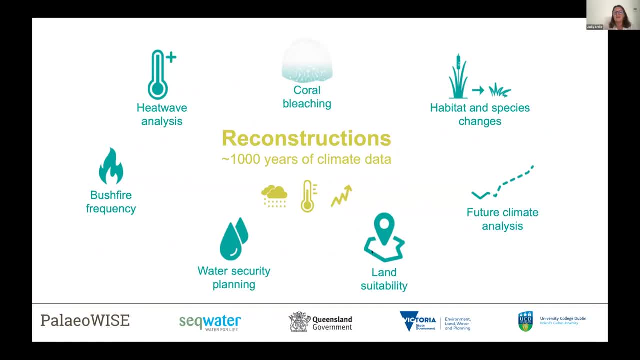 used in heatwave analysis, bushfire frequency, you know land suitability, obviously, future climate analyses, habitat and coral bleaching, You know. once you have that time series, you can start looking at these changes in a number of key aspects that are now very, very relevant to Australia's future. 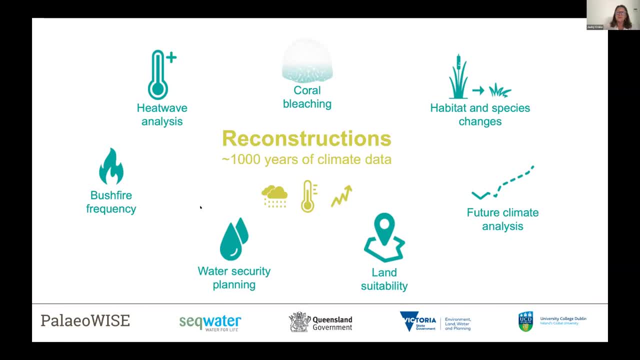 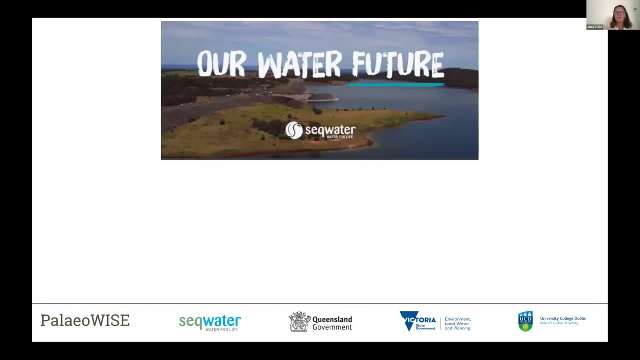 adaptation to a warming climate. What I want to focus on today is just some very brief applications to water security planning. So obviously, as I said, SEQ Water are, you know, the major bulk water supply authority here. They're completely responsible for the supply of both our drinking. 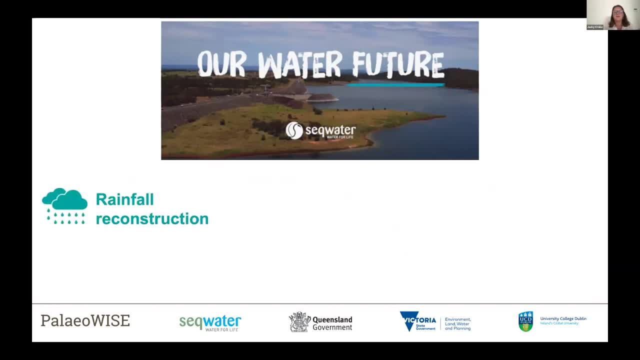 water, but also water for irrigation, supporting agriculture. So one way that they would use these reconstructions is in their rainfall runoff models and the water resource assessment models. So this is work that John Vitosky has done, which is a kind of a. 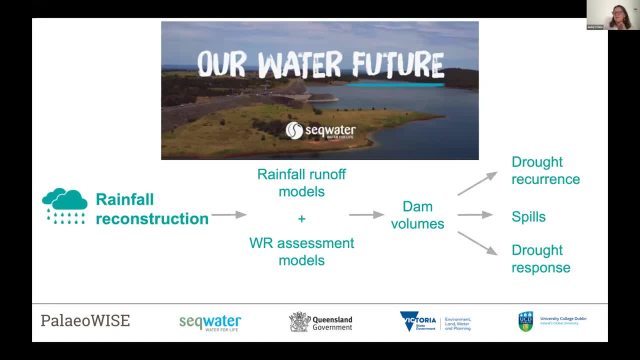 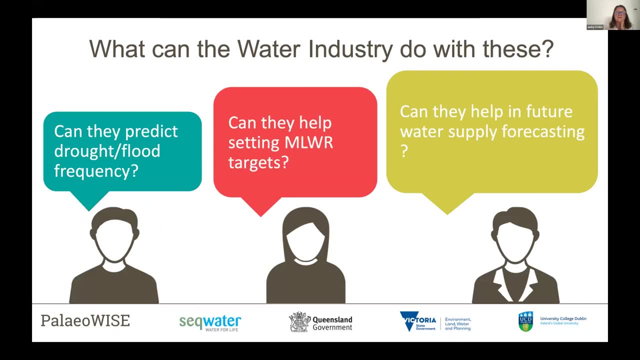 standard work that he does, And he's done it in the same way that he does this work for SEQ Water anyway. This allows you to look at things like dam volumes, but also drought occurrence and, you know, spills and so on. So how can we use this information to better predict? 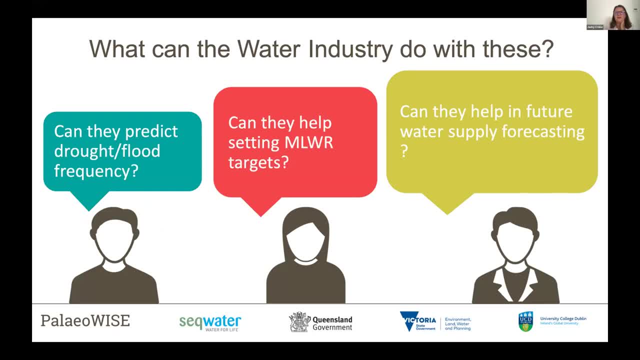 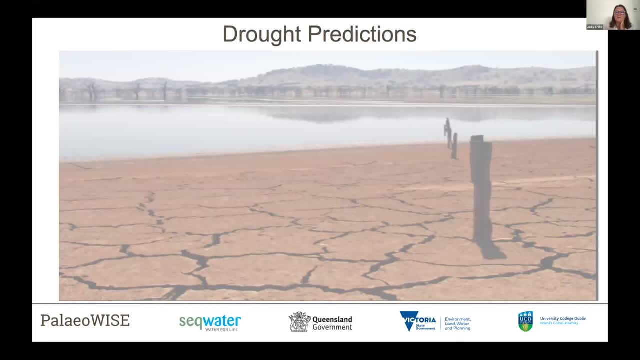 you know droughts and floods frequency. Can they help with things like you know water level restrictions and how do they actually help with planning for water supply scenarios? We've obviously had several major droughts now in Australia in general: the Millennium, the Federation drought, which really just highlighted how vulnerable but large parts of Queensland are almost permanently in drought. 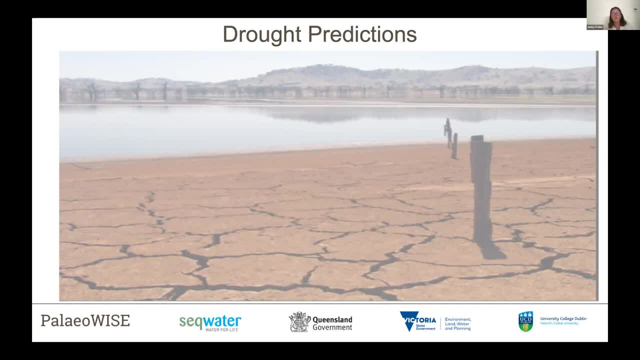 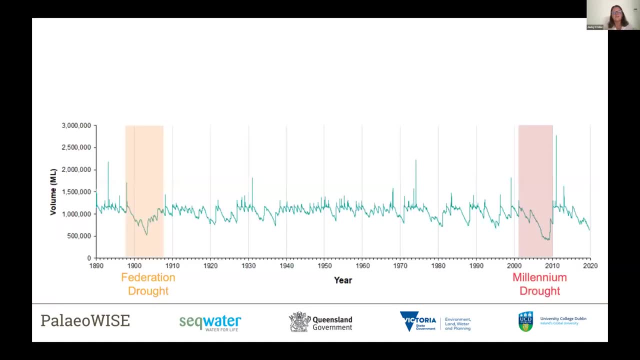 Prior to the recent rain in 2022, SEQ water's major dam storage, Wyvernhoe, was sitting at around 36%, So we are completely aware of the vulnerability in this space. So what John did was he did a simulation model using his water resource model- I think it was a combination of Sacramento in this case- and he actually tried to quantify the dam inflow for those two particular droughts. the Federation that we have here, you can see, and the Millennium. 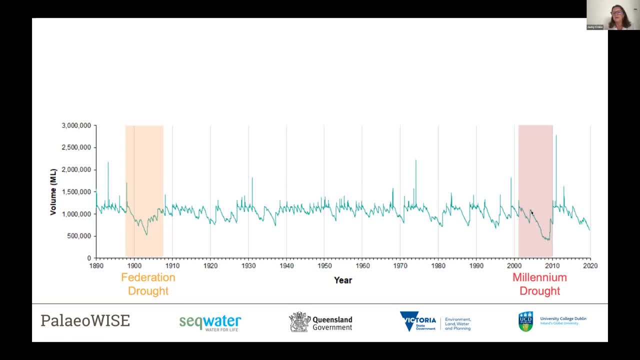 And you can see just basically the slightly different sort of drawdown characteristics of those two droughts. but the main purpose here was that we would get an estimate of the volume of water that was characterized with that, which turned out to be about 450,000 megalitres. 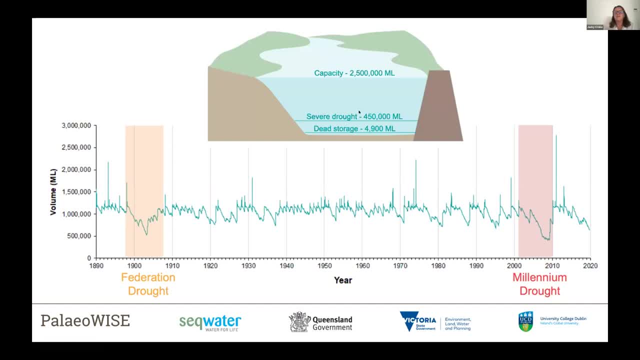 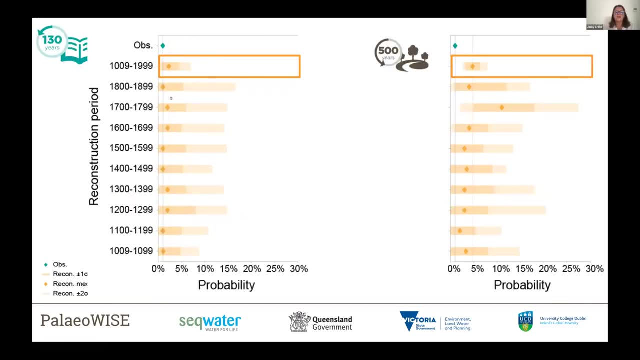 So we've estimated that a severe drought would actually occur at around that threshold. So what John was able to do then was he ran two scenarios. So on the left of the screen here you'll see what's known as the static climate model. 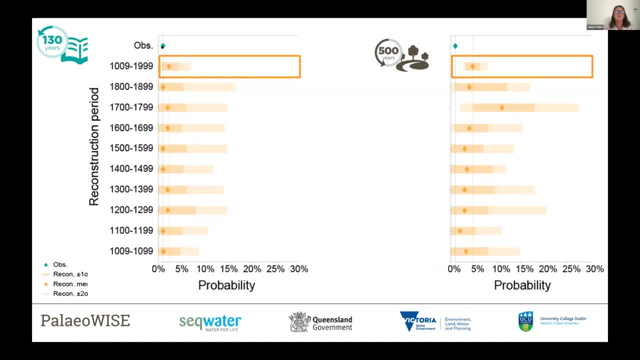 There's no variability. This is the prediction here for the inflow. It's about 450,000 using just the observed records. so it sits at about 1%. if we use the entire records, the thousand year reconstruction that increases to about two and a half percent. 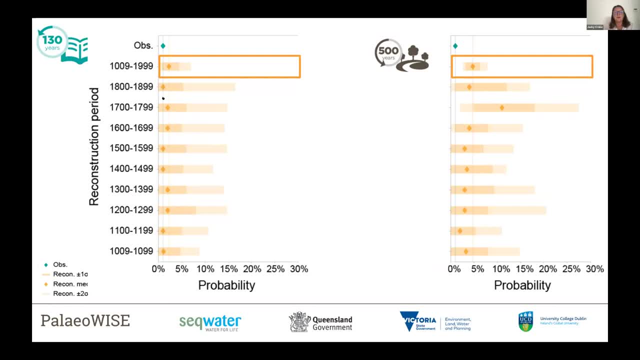 But you can see that the impact of that static climate model is there's very little variability in the centuries throughout that. If you look at the paleoclimates time series that John ran- this is the observation prediction here- But you can see for over a quarter of a century there's very little variability. 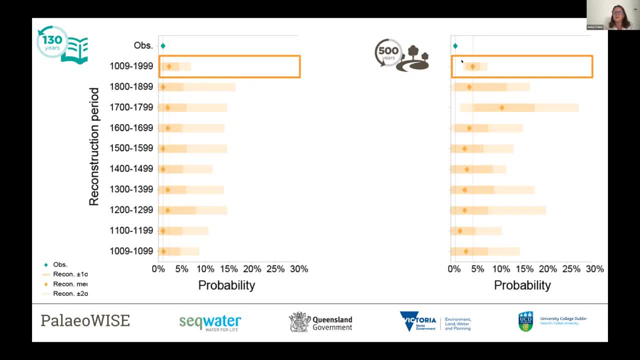 But for that one thousand year time scale the annual exceedance probability has increased from about one percent to five percent. The advantage as well is that we can actually look at the performance. for example, in that 17 hundred you can see that the probability is actually increased to maybe about 10 or 12%. 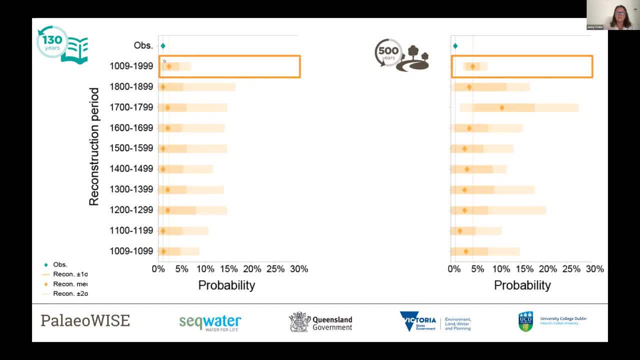 So for Seq water, rather than looking at a standard estimate of the probability of that water becoming more severe, of, say, a millennium type trace sitting at around 1%, we can actually sort of inform them that in fact the probability of that is much greater. 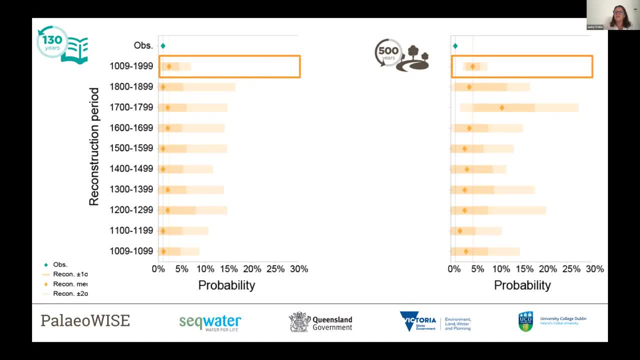 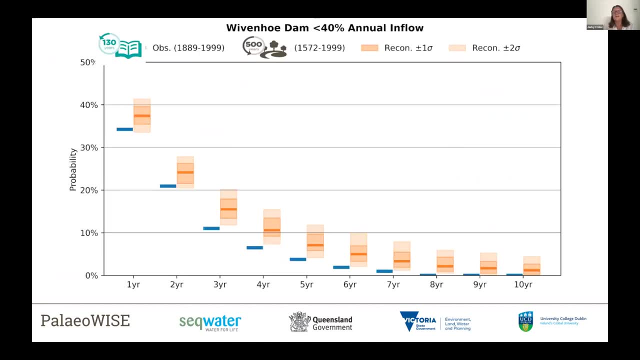 It has increased with that thousand year record to 5%, but it can be up to 10 or 12% if you experience a century, like we did previously. All of these outputs are really just to demonstrate the difference between using the historic, the observational period alone. 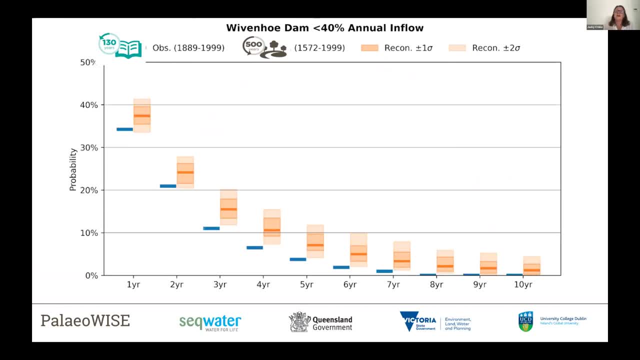 versus using that longer time series. This here is annual inflow into Wivenhoe Dam, for example, and each of these boxes which is sitting above the blue boxes, over the multi. so Wivenhoe is a multi-year storage dam. You can see that the probability of that particular inflow 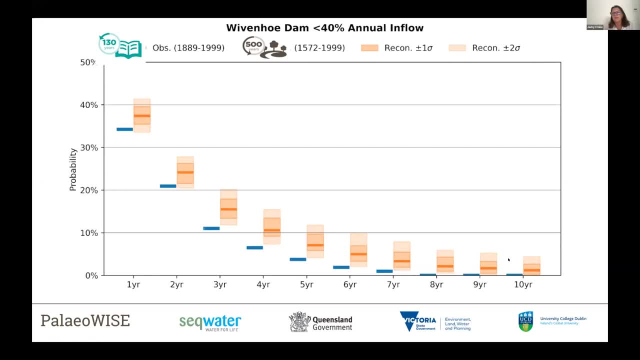 over that timescale is always higher, So even at the 10 year timescale, but, importantly, when we're using water over that five to six year timescale storage using one data set. the Wivenhoe Dam has become the state agent. 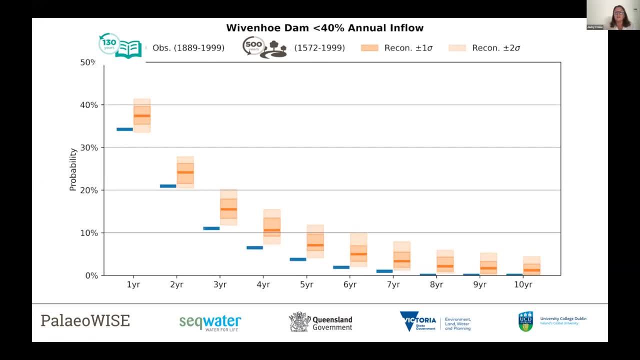 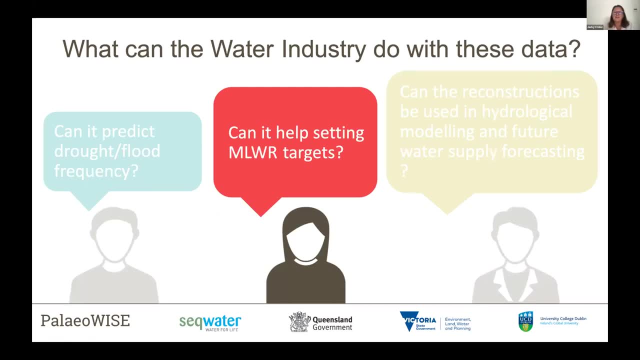 for thatienstagedenden development. For those that used those key data sets that I said that this is an operational data set along. The other area that SEQ Water are particularly interested in is the setting of medium level water restrictions. Many of us living in Queensland 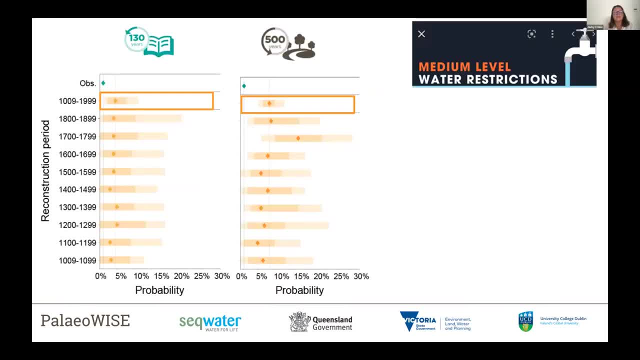 are very familiar with when these kick in, but to a certain extent, you know, using that longer time series. So the same output here. for example, using the Static Climate Model model and the observational period medium level water restrictions are a very low probability. 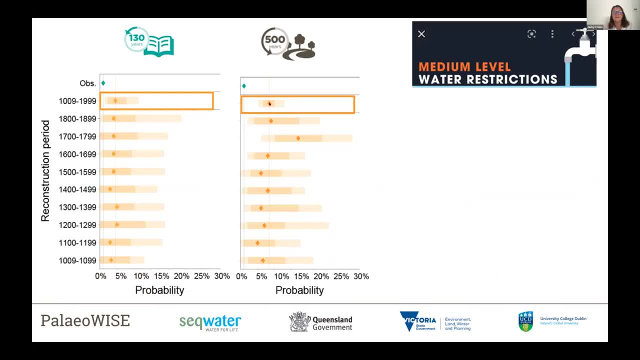 If we start looking at the longer time series, we can see that that probability is actually increased from about 4% to 8% And we can start to see some of the variability in some of those centuries. So, in terms of them, managing the timing and the preparation, the preparedness, 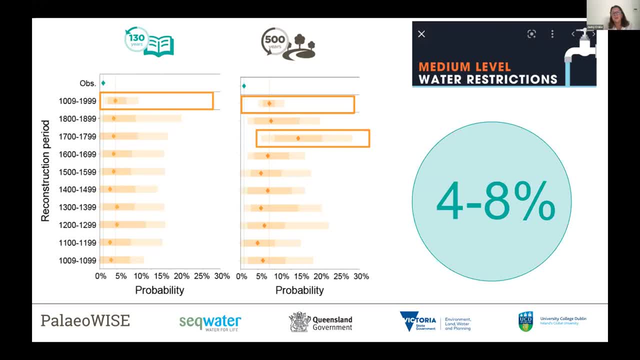 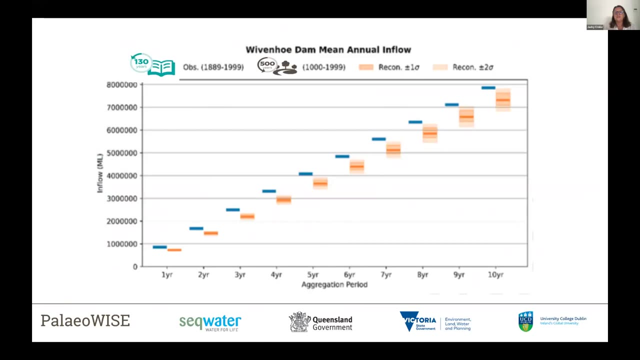 for these sorts of events by showing them the impact of some of that longer time series data you know they can start to better inform, they can start to make you know more informed decisions around. what point would they kick in? Other aspects would be, as I said, the mean. 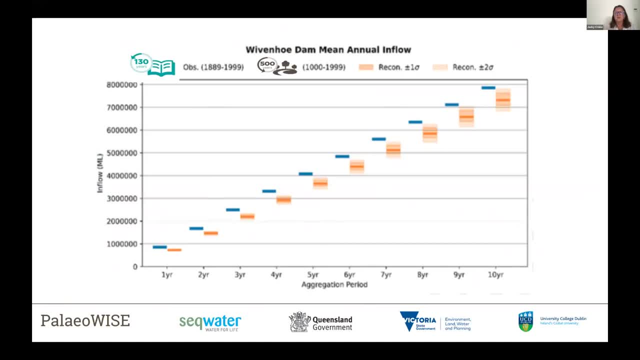 annual inflow. Again, this is a simulation using the water resource model that John did And we can start to see that because that reconstruction period was overall it was actually quite a dry period, the probability there the inflow is actually reduced significantly in some. 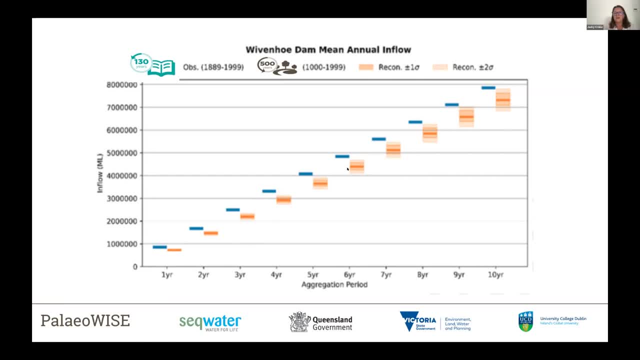 cases here. but over that time period of the aggregation period, And what this informs SEQ Water is that obviously relying on these estimates, just using the historic data you know, obviously operating within these 95% confidence intervals would allow them to better manage the. 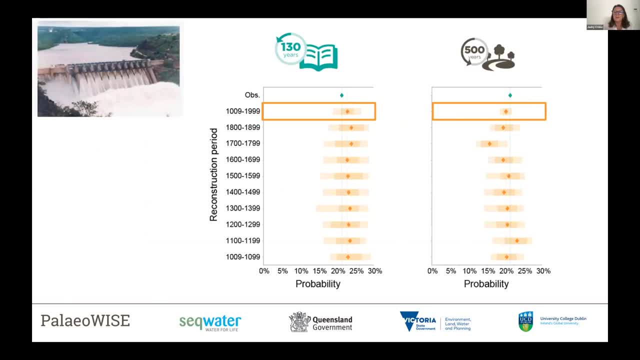 risk of drought, And the same analysis can be applied to dam overspilling, Irrespective of the output. here the whole logic is the same. Once we have an observation period of 100 years, once we change that to 1000 years, we can start to see. 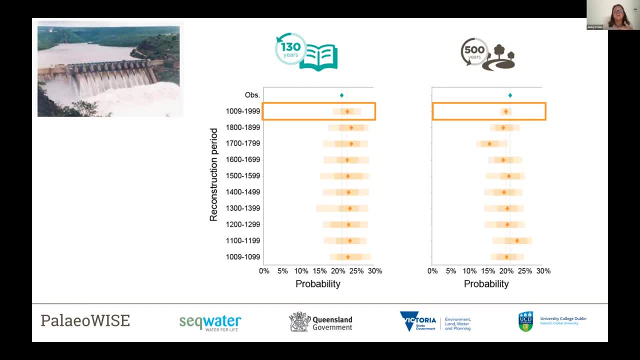 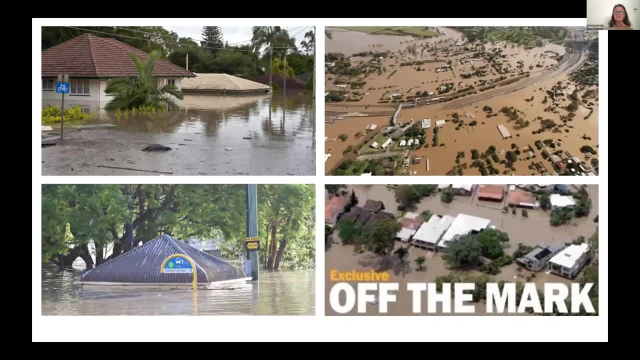 fairly significant changes actually in the probability of an event, whether it is a drought or a water restriction or a dam overspill- actually occurring. One of the things that people have asked us is coming back to the extreme flood events. you know to what extent is the 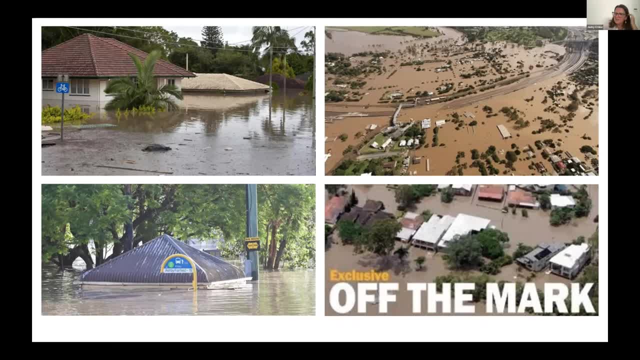 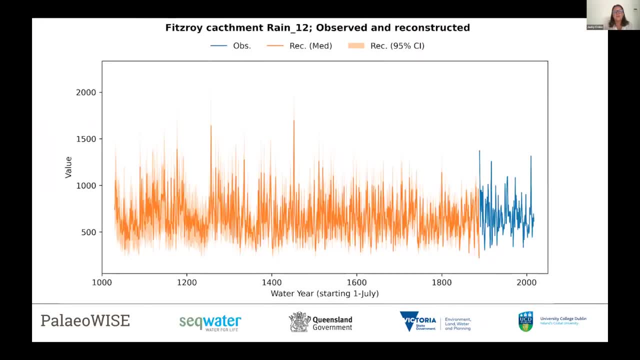 time series actually accurately predict the magnitude of these. So the time series, as I've shown, you can identify. you know periods. For example, here we have the Fitzroy catchment. This is the time series. We can clearly see that there have been years where the rainfall estimates have 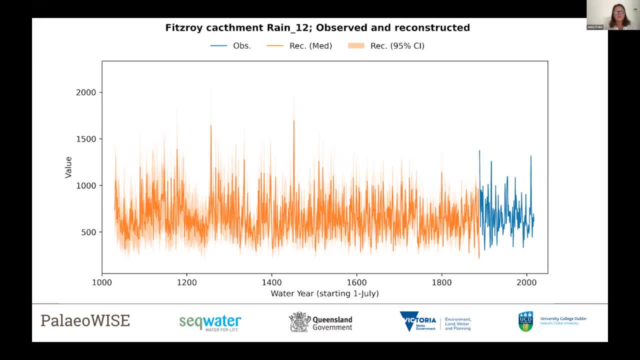 been. you know several. you know orders of magnitude. well, not orders of magnitude, but much, much higher than we observed in the observational period. In fact, for this record, there are at least 25 years in the Fitzroy where we experienced rainfall. that was beyond that ever. 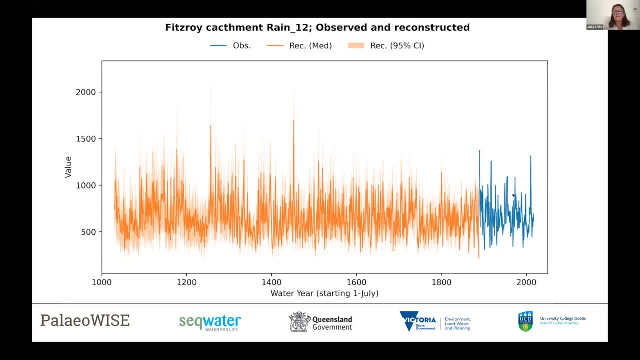 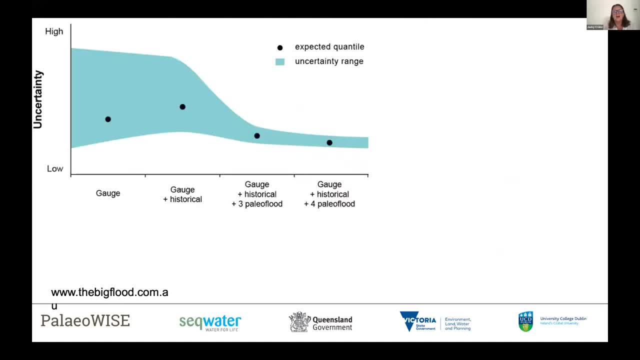 recorded in the historical period, So we do know that there's been some more extreme flood events. In terms of using these time series to predict magnitude, we would advise against it, simply because the resolution just isn't there. It's what we demonstrated in the big flood project was. 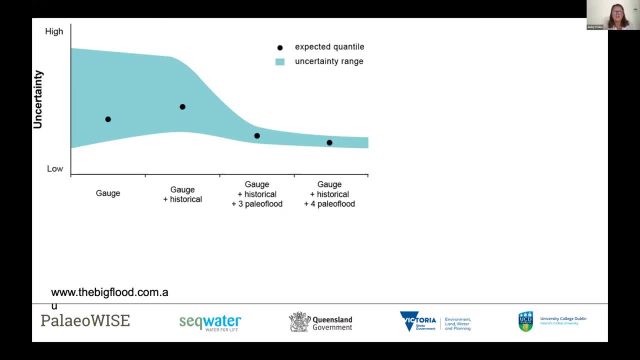 that you can use a different technique- paleoflood reconstruction- which is now well established globally. But Darrell Lamb in his PhD as part of that project, demonstrated that the degree of uncertainty around just using the gauge data for the prediction of 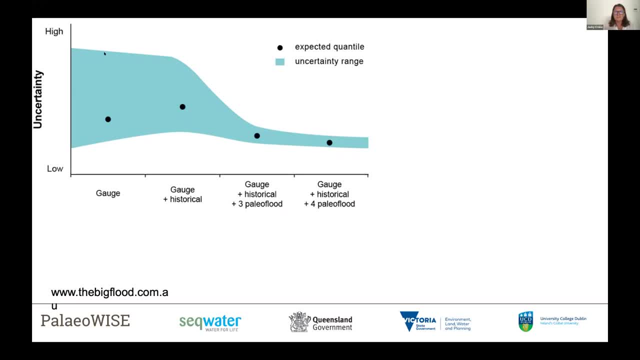 these extreme events was considerably high. as soon as you added in the historical, that reduced somewhat. But basically as soon as you started to add some paleoflood data in there which very specifically measures flood magnitude in addition to timing, you can actually reduce that uncertainty by anywhere up to 60 or 70 percent. 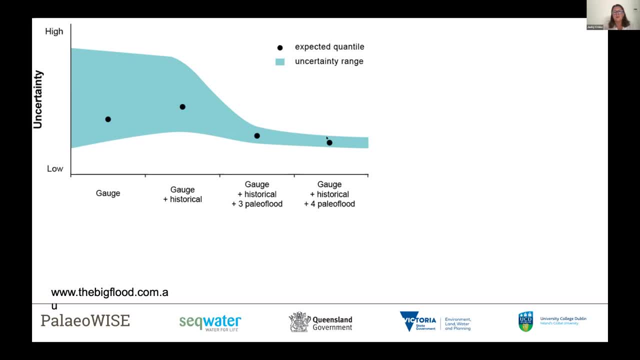 This is not a very complicated or indeed costly approach, So we would certainly advocate, if particular stakeholders were interested in the detail of elevation, of flood magnitudes and so on, that this would be the approach If you're just interested in using rainfall to run your water. 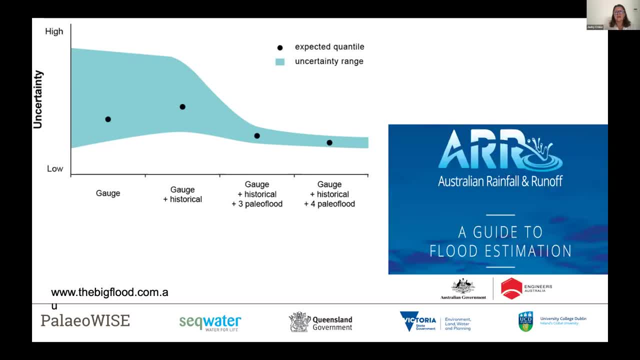 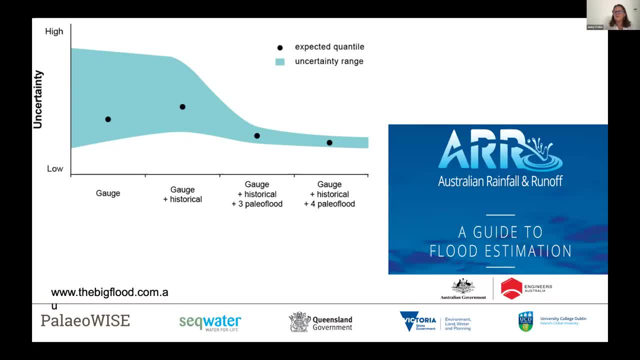 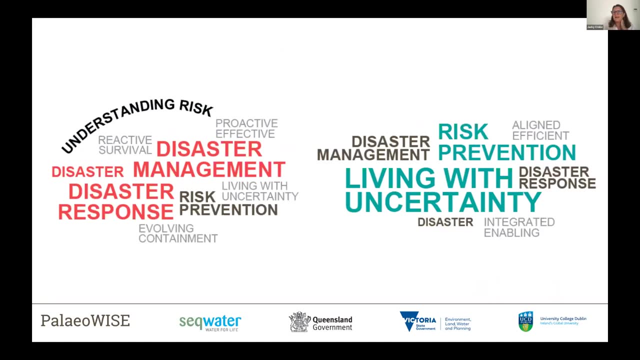 That work included now in the Australian rainfall and runoff updated versions where it is recommended that paleoflood analysis can be used in the prediction in the intensity frequency duration predictions here in Australia. So that was a bit of a whirlwind, Really. everything that we've talked about here is hoping that these data sets can actually assist. 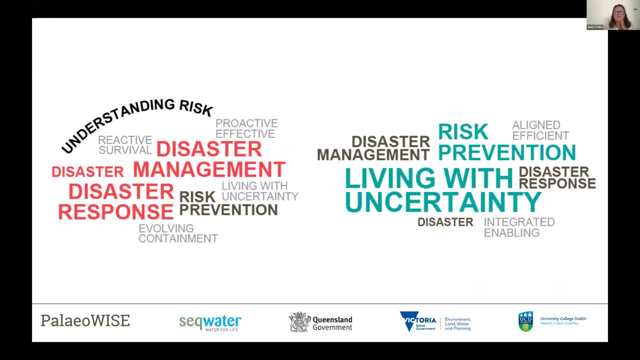 everybody. There's a vast range of stakeholders that are engaged both in risk and disaster management, this aspect of living with uncertainty. you know there's been a lot of conversation really following the events in 2022.. How prepared are we, You know? should we putting? 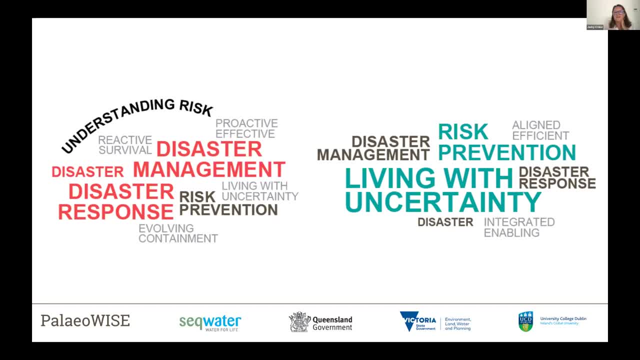 our communities at risk of some of these extreme flood events, And what can we do better? So we're very keen in this project to make sure that the information is reaching as many of those stakeholders as possible. And we're demonstrating. we'll be producing a series of infographics. 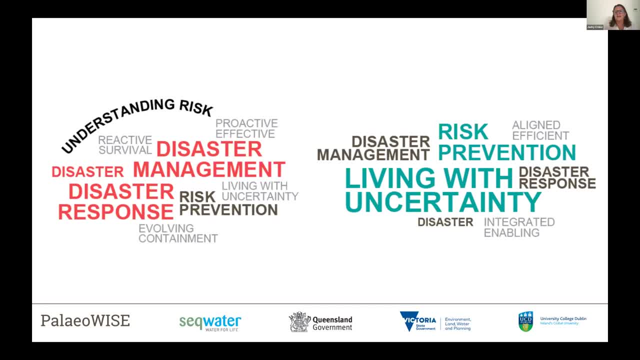 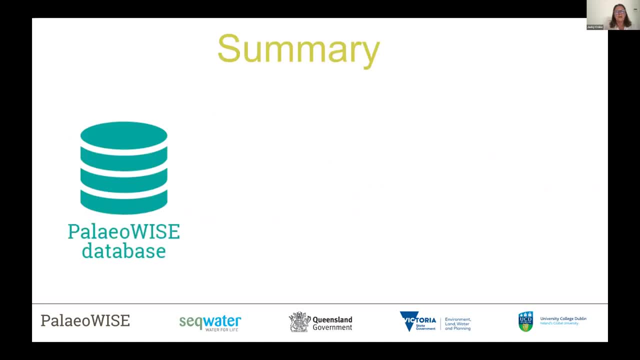 demonstrating some of the potential of the time series to help in some of that sort of climate adaptation work. So just to wrap up, I gave you a brief introduction to the PaleoWISE database that's freely available now on our website. PaleoWISE-R is the approach that we use. 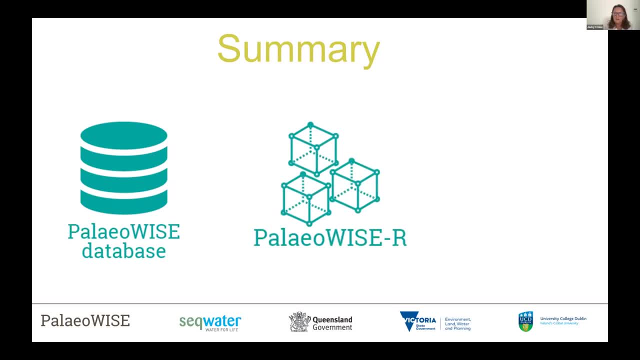 to reconstruct climate variables of interest. In addition, we used it to reconstruct major climate drivers of interest. We've demonstrated a couple of the primary outputs in terms of the time series, plots and some of the things that you can do. Obviously, the specific application of the time series or 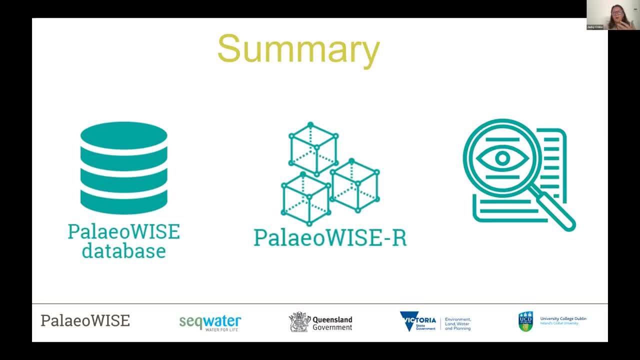 any derivatives is really user dependent. So we can't produce a definitive application here because, in all honesty, every user- potential user- would have a different need. It would be trying to answer a particular question, for example. So we've demonstrated a couple of the 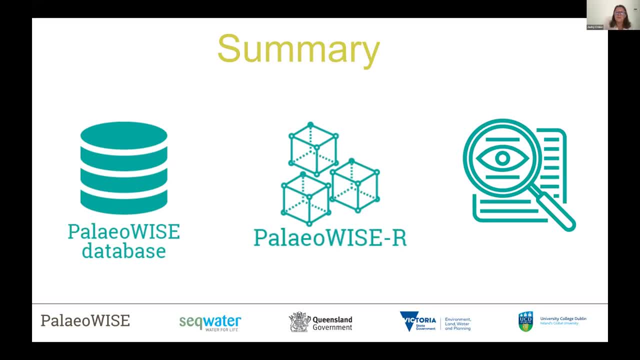 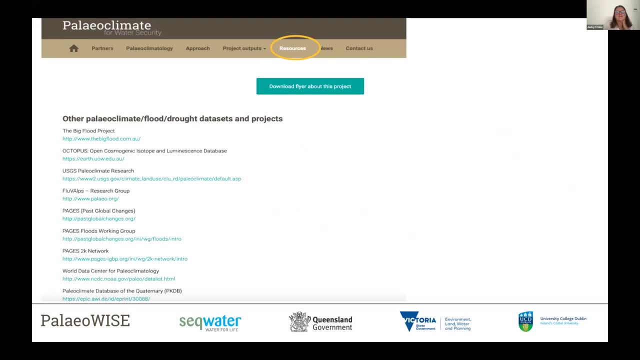 things that we can do. So really, it's up to the individual user, but we've done our best to ensure that the data is as freely available as possible. So, as I said, the Paleo Climate for Water Security website has all of the information that I've talked about this morning. There's also the 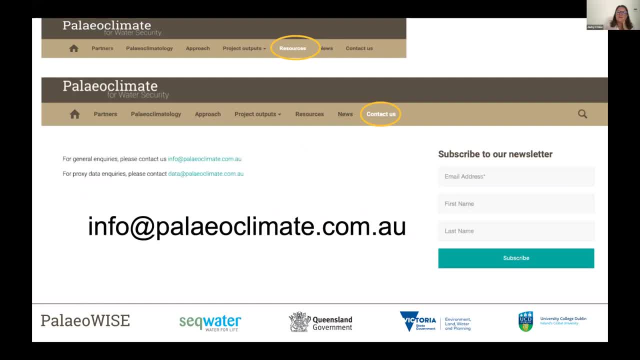 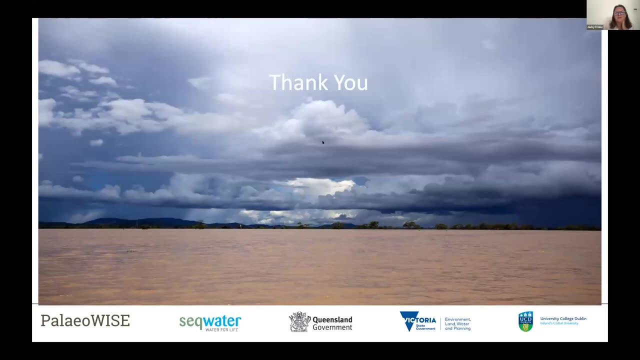 opportunity to sign up to our newsletter so that when new additions are added to the website or we publish any new papers, that's also available. So feel free to hop on there. Hopefully I've left enough time to answer some questions, But thank you very much. I'm hoping. 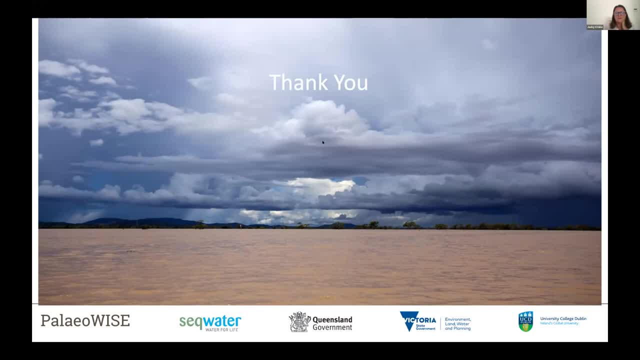 that that overview, as rapid as it was, gives you some indication really of the potential and indeed the enormous value that these data sets hopefully will have to future predictions. So I might leave it there and see if there's any questions, I'll stop sharing my screen. 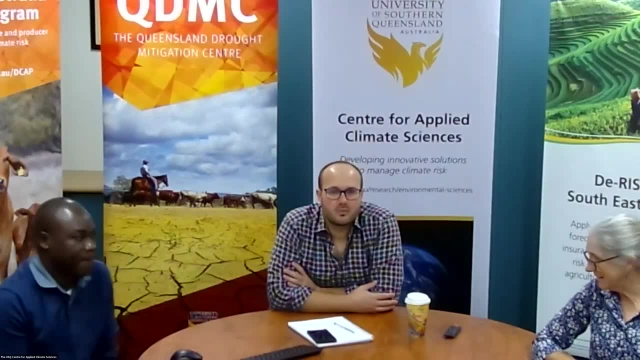 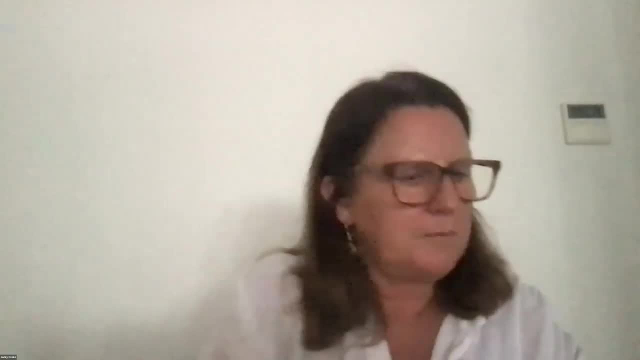 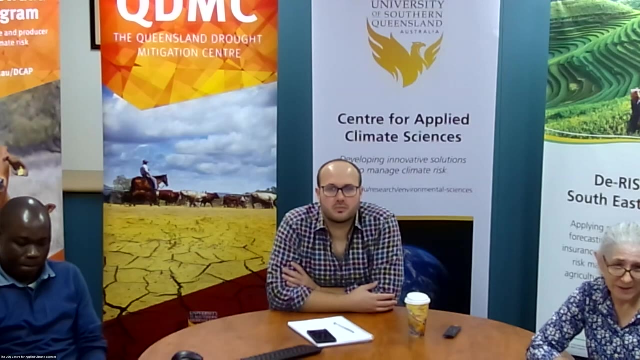 Thank you, Jackie. Do we have any questions? None currently listed in the Q&A. That's okay, I guess just listening to you. So obviously there's a good relationship for rainfall. Do you find relationships also for temperature, and particularly sea surface temperatures? 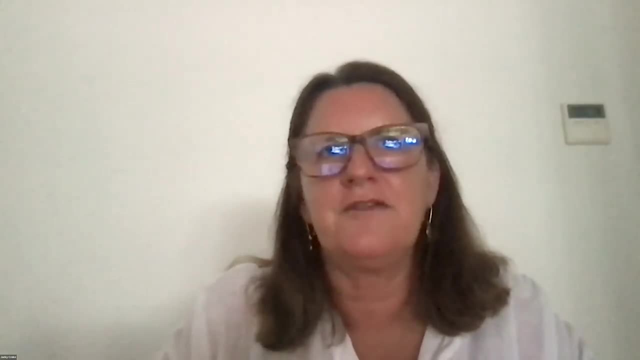 Yeah, to be honest, Catherine, we haven't really. you know, given the size of the database and what we were actually sort of focused. Yeah, we had to narrow it. You know. I put it out there If anybody is interested in looking. 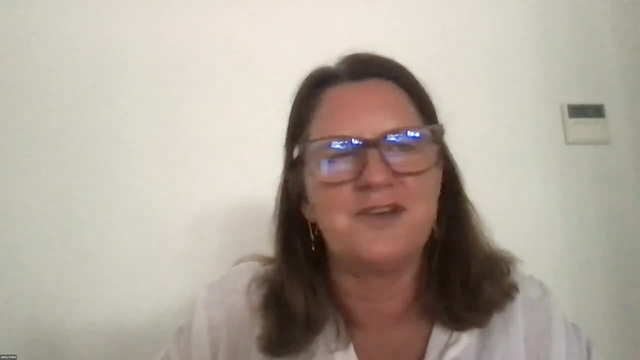 at the temperature database in particular. I would certainly welcome that collaboration, But at this point the reconstructions are there but we haven't really focused on them in any way that I could give you any further insights. We've really focused now. 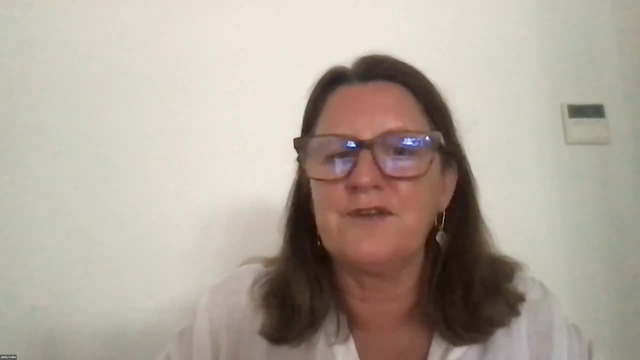 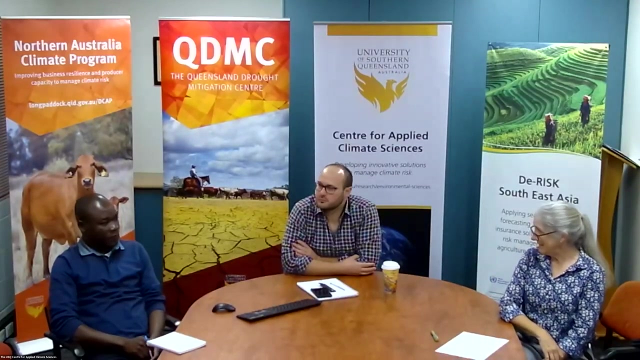 given the emphasis on floods and draughts, we focused on rainfall, SPEI in any of those other derivatives. you know the extreme floods and draughts. Otherwise it was pretty overwhelming. Yeah, absolutely. Does anyone in the room have a question? 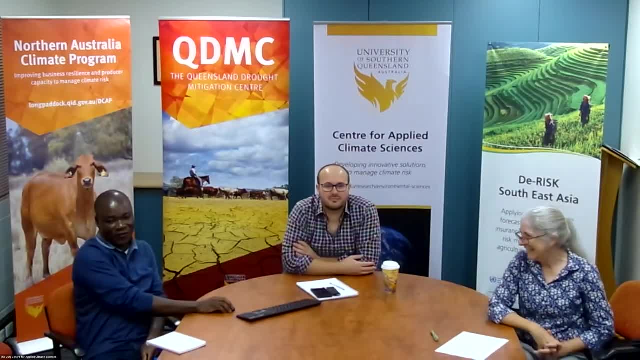 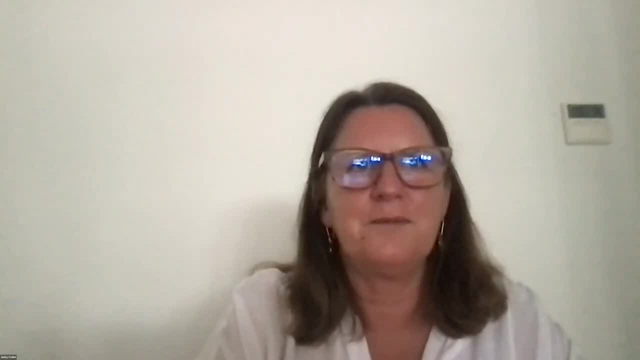 Louis does a lot of crop modelling. You might be able to incorporate some of that into it. Yeah, I guess that's one of the potential applications. that we're hoping is that people you know may see the application of some of the time series into crop modelling. Spoken with some 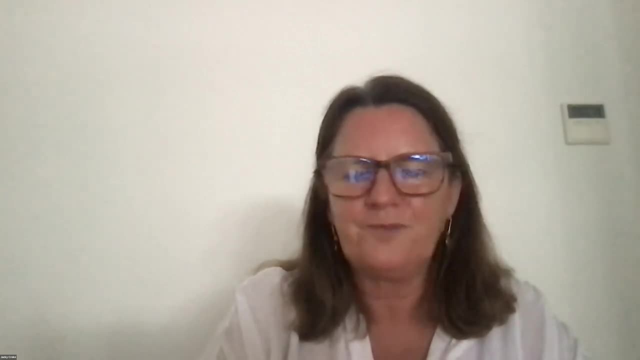 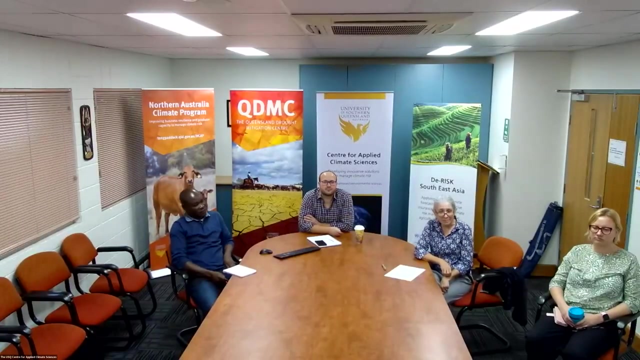 of the collaborators at DES, for example John Carter and others. Again, it would be great to see the Yes, the crop modelling and the pasture modelling. Pasture modelling- yeah, that's right, It would be. you know, it would be very useful, especially those periods when. 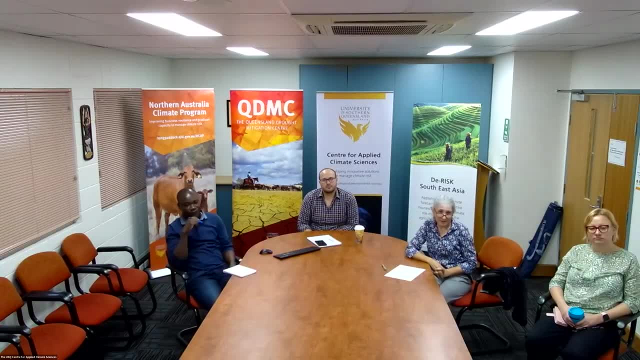 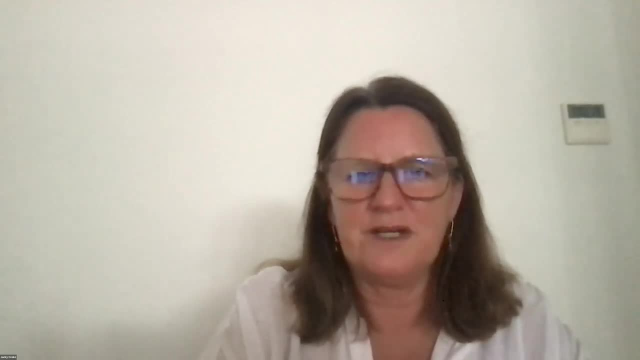 you know if it is likely that we might see some of those higher rainfall events again. Absolutely yeah, that's right, And I guess these are all conservative estimates really, which I guess in some respects is potentially alarming for us, But nonetheless they are conservative because of course we don't really have 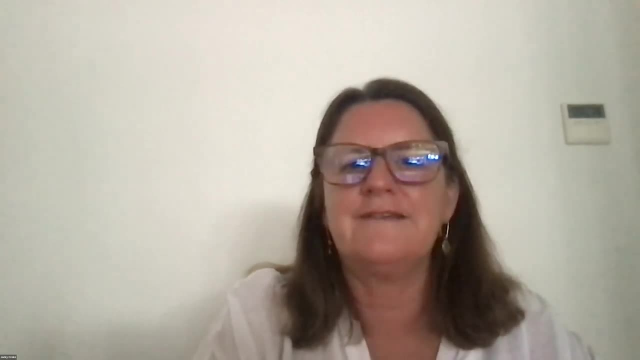 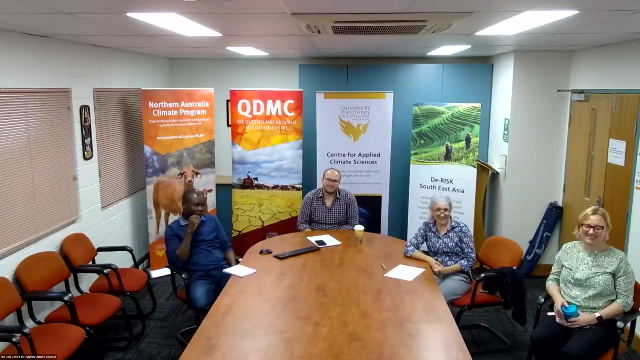 you know, urban or human influences to a certain extent as we have in that historic period as much. So yeah, I'll hand over to Christina. Hi, Jackie, Great talk. It was really interesting. I was wondering I'm not working in this area. 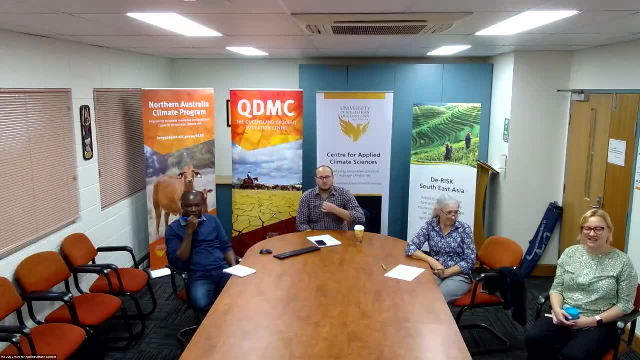 so pardon my naivety, I guess, But I was just wondering, like I read that for the like the 22 flats, So we just had. So, similarly, like the data was there but the governments are now taking it on board and using it to. 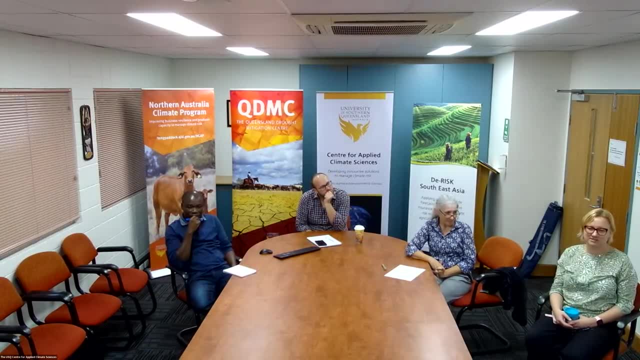 you know, warn the people properly and in advance. So I saw that, yeah, there were. The predictions were like a month or two before those went, like the recent floods were Queensland, but it was just not acted upon. I know it'll probably be on the scope of your research, but I just thought: what's your thoughts in terms of? 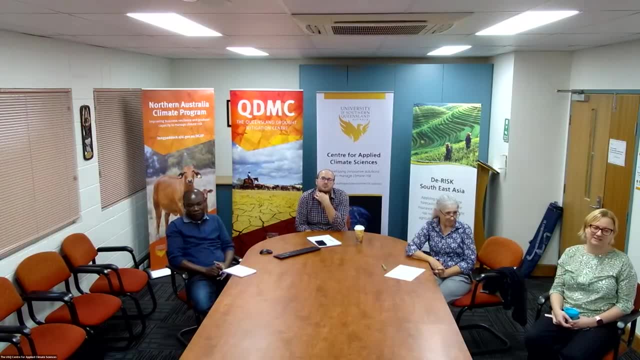 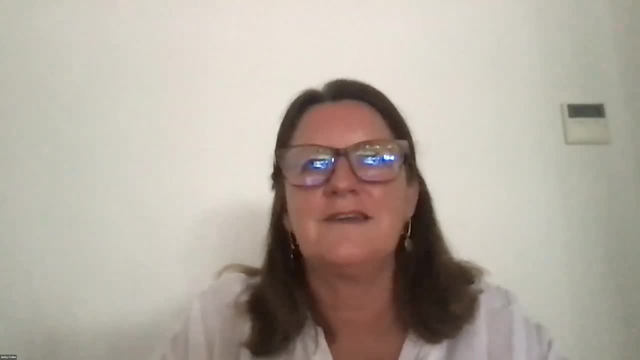 how can we get the governments to use that data like more efficiently to actually have a? That's an interesting question, a more efficient way to actually have a look at it, have our own ground, you know, benefit for people. yeah, it's a big question, isn't it really? i mean, 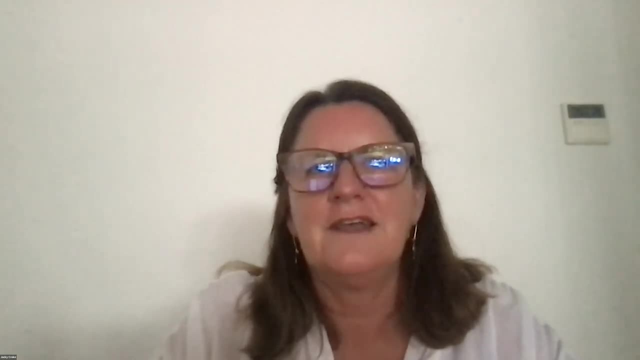 i think australia's focus has been to really fund, um, you know, flood cleanup, flood recovery. really, that's where the investment, the financial investment, has been. i think there's probably been much, much less gone into flood warning and you know flood communication and i know you know many, many people here in brisbane were very, very disappointed with the absence of any. 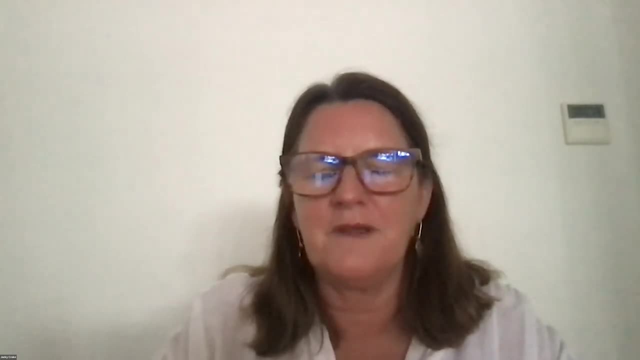 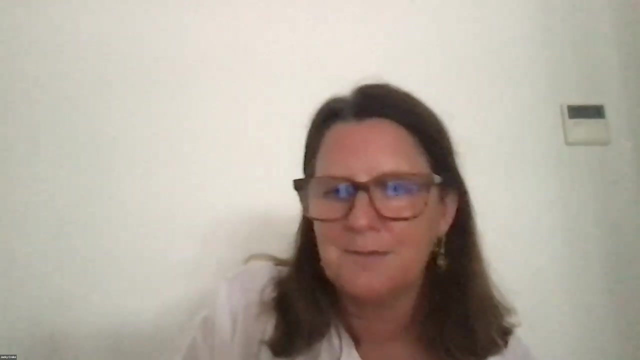 warning really, around those, those floods, particularly in some of the upper creeks, and this, that that came out of 2011 very clear as well. there simply wasn't the infrastructure in place to be able to communicate that. um, you know my- i guess one of my- personal frustrations. 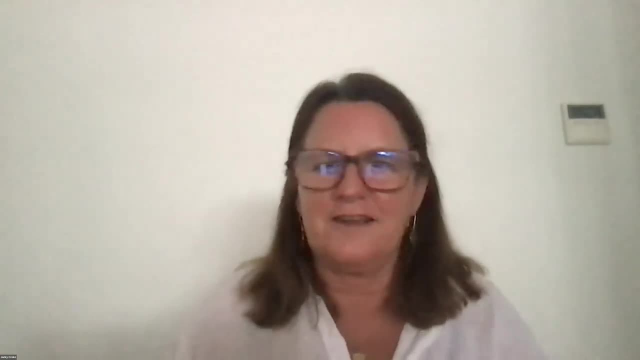 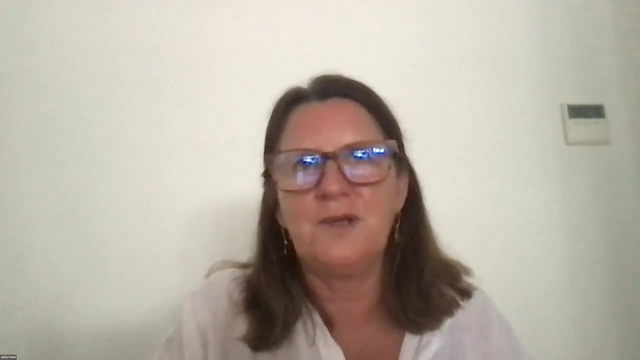 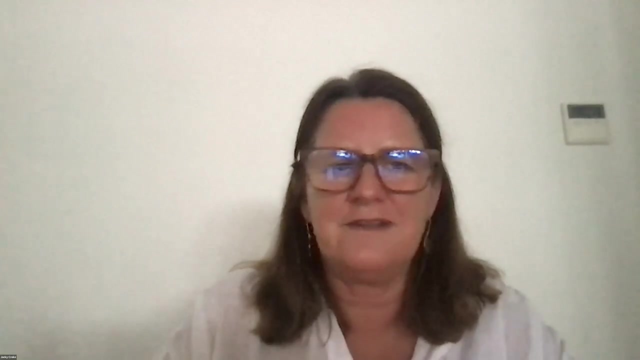 getting it into. uh, you know, fairly obvious users like seq water or um, you know the bureau, for example, that's, that's a major challenge because really the incentive to do that is there's very little from their perspective really. uh, i don't know whether that's going. 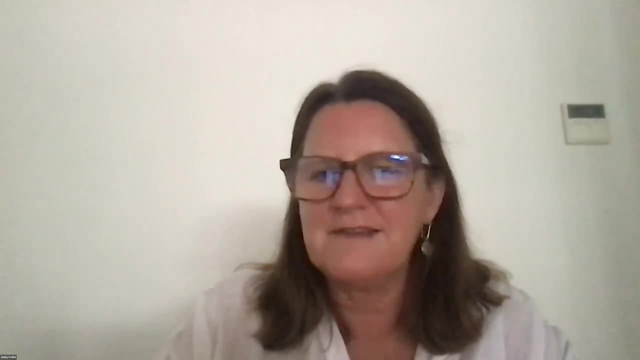 to change? i hope it will. i think the frequency that we're going to experience these floods may well, uh, change the focus of you know sort of clean up to you know better predictions in my case. why wouldn't people use that data set? it's a, it's a if we're going to, you know if we're going. 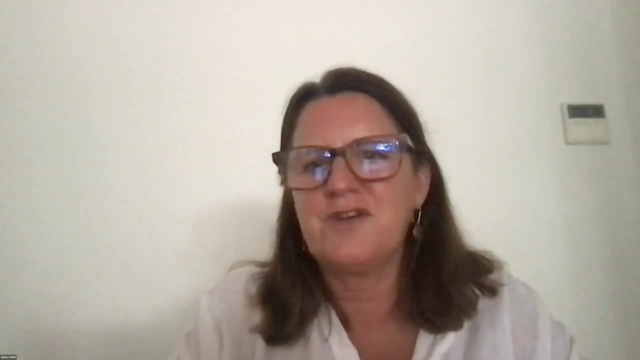 to stress, test, uh, both our infrastructure, but also where people are living. why wouldn't we use a longer time series that actually has uncertainties quantified, like if i'm a person living on a flood, i would like to know, you know, within the confidence intervals am i going to be flooded every you know? 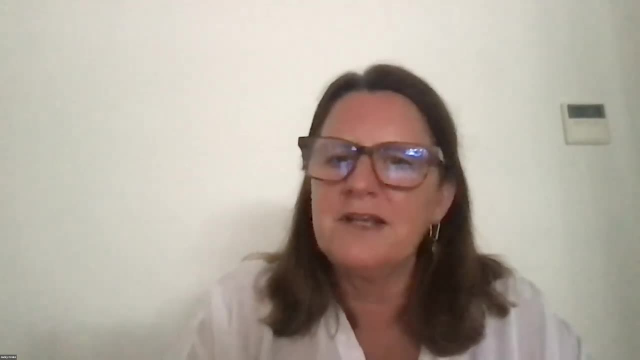 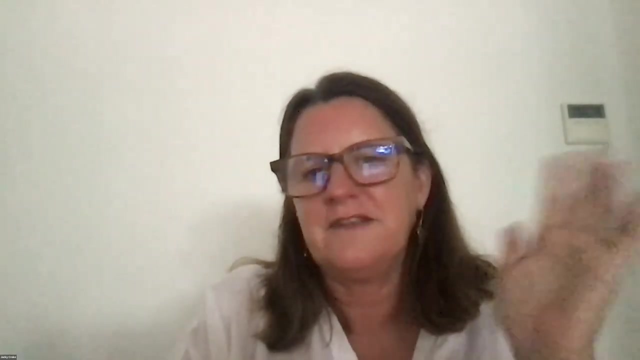 year now, or 10 years and so on. so and we can see from some of the output that i showed you just using that observational period effectively shows no variability. they're not modelling change. they're not modelling for change. when we look at the longer time series, we can see that there. 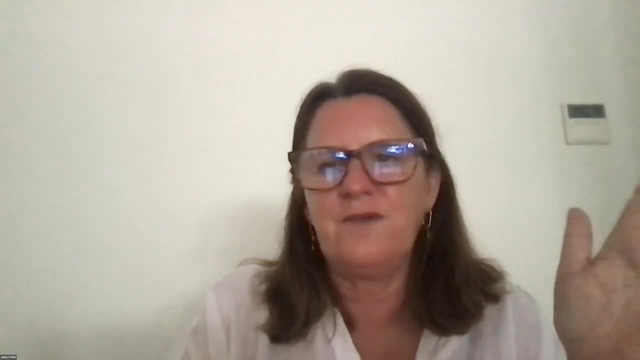 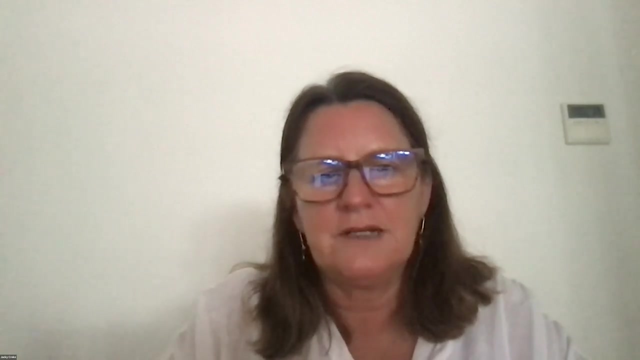 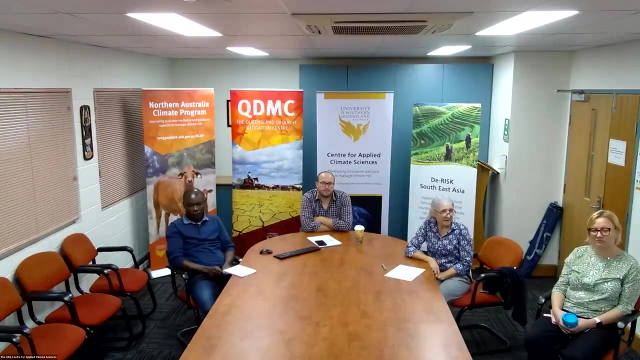 has been significant variability, even outside of you know, more recent climate change, for example. and how prepared are we for that? um, and i would argue, probably um. you know, we need to be need to be focusing better on that, capturing that variability. jackie, what was the response of? 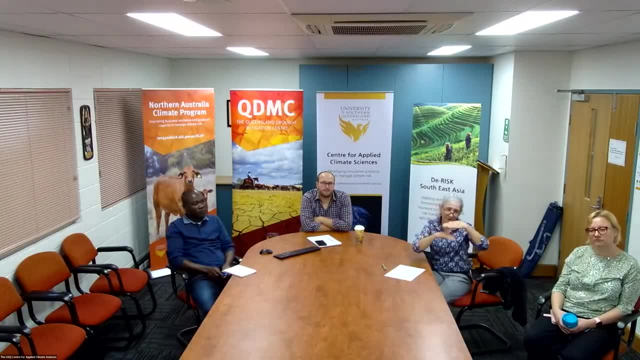 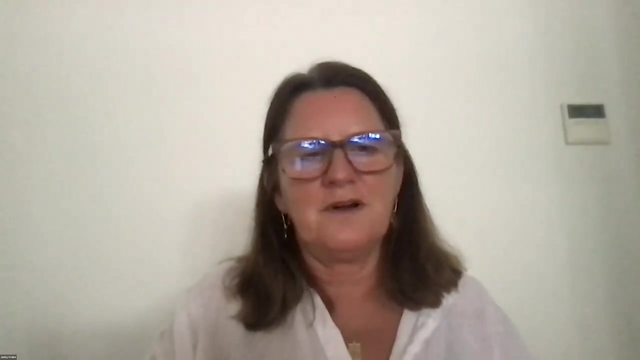 seq water. i mean i you've spoken about the, the modeling, in terms of how it informs drought water management, you know, heading towards drought um and the introduction of restrictions, but when you showed them, the reconstructed data that showed these more extreme rainfall events, yeah, i mean, to be fair, seq, seq water are? you know, they've been a very um good supporter of this work i have. 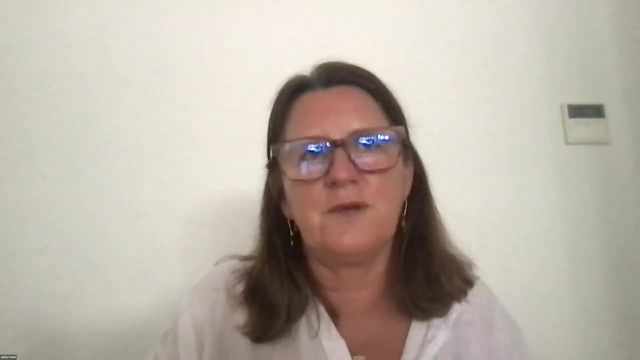 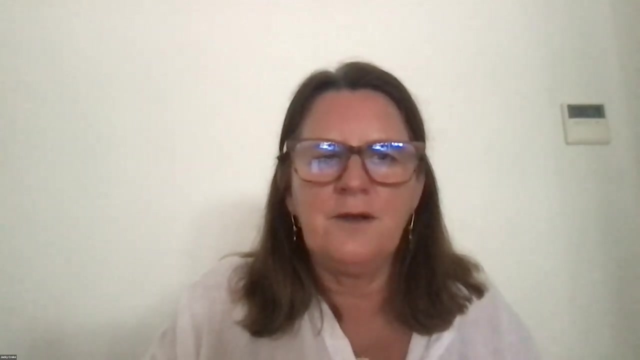 to say they've, they've invested in it and they've been very supportive of this work and i think they've invested in it, and they invested in the big flood event as well, um, you know, in terms of generating that research understanding around these extreme events. i think you know obviously. 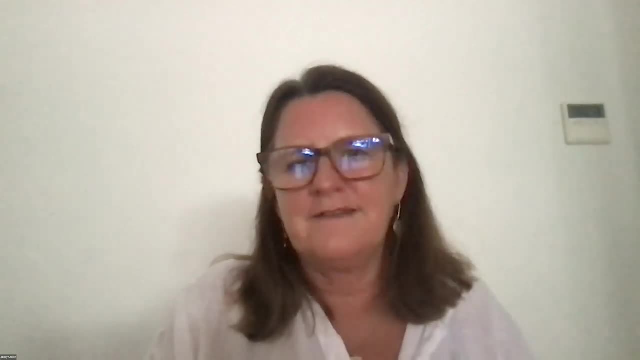 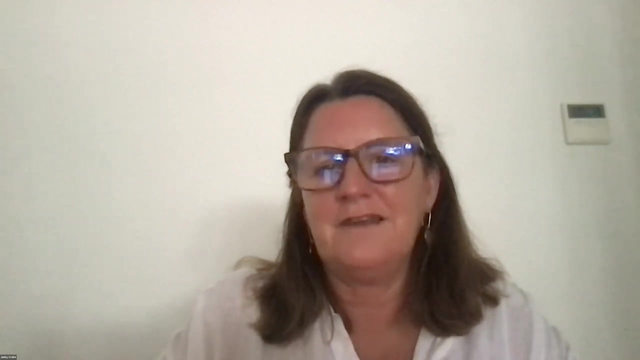 everything is is a reactive. it's a reactive space, you know. so it's about giving people time. you know, i've now concluded that this isn't going to happen overnight. it's going to be a case of, you know, trying to maintain awareness of the data sets and, you know, hopefully those collaborations between 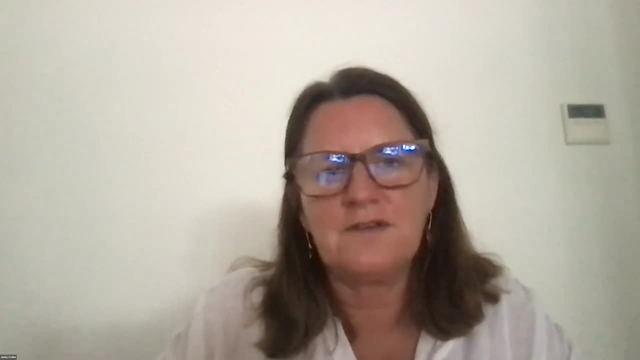 uh, the water modelers. you know, john vitosky does all the water modeling for seq water, so john's been a collaborator on this project and that's been enormously valuable for us because john can see what are the applications, what are the limitations. you know what sort of resolution do you need to be. 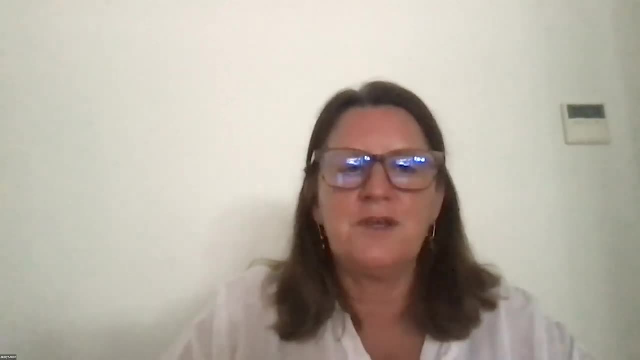 able to do the sort of scenarios that john would do for them. so i think that's been hugely beneficial and you know that's been a huge um win for the project is just having that collaboration. so i think it's it's hard to say, i think it's hard to say. i think it's hard to say. i think it's hard to say. 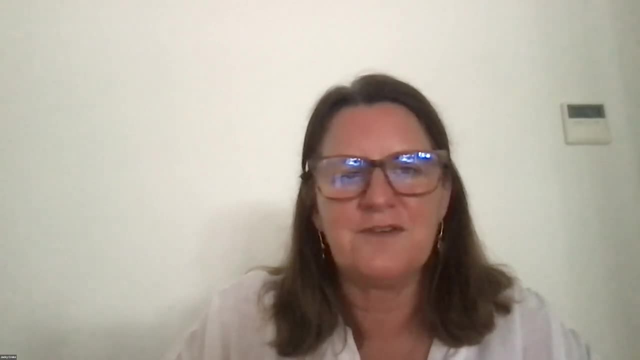 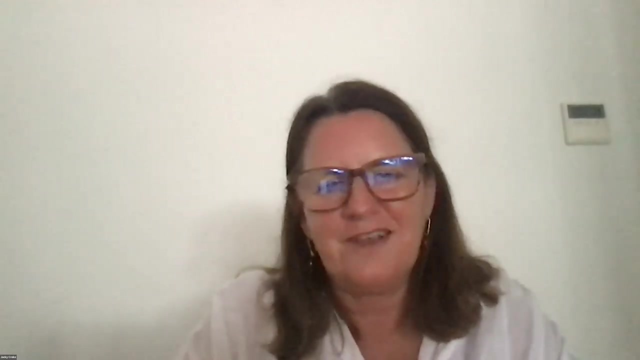 it's hard and, as you would know, i guess, um, from my perspective as researchers on the project, a project has a start and an end date. you know, unfortunately, this project is now ending. uh, the extent to which we'll get future funding to keep you know, raising awareness or keep you know. 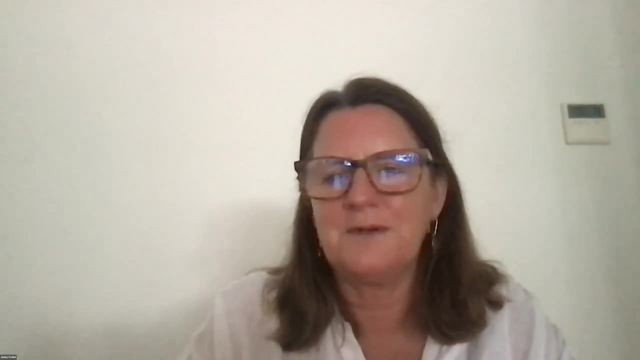 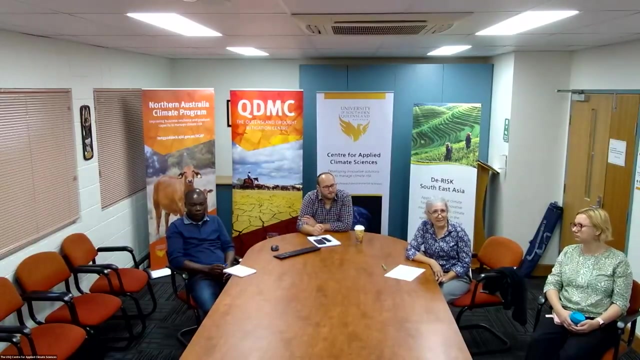 collaborating is is very uncertain in this, in this space as well. so it's it's definitely um at both ends of that spectrum, i think i imagine there's a little concern, though, about you know what, whether the infrastructure which is based on the recent historical inflows, um how that would cope in. 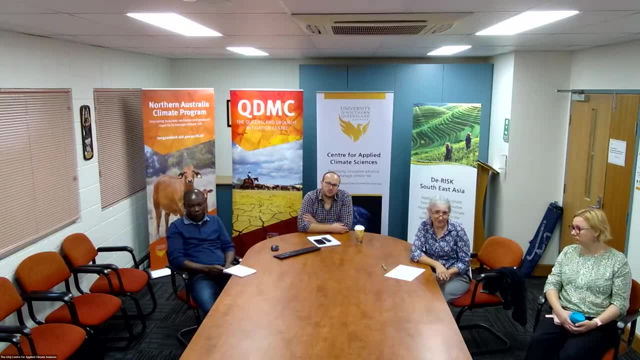 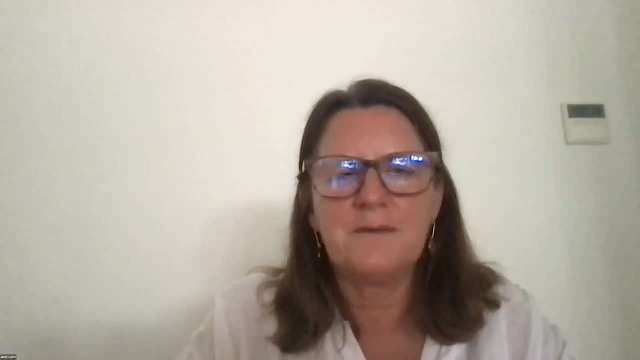 those situations, given the challenges already that we've experienced with extreme rainfall events that we have experienced recently. yeah, i mean seq model would be modeling there for pmf. uh, you know, there would be modeling basically for very high, uh, extreme events, anyway, like a one in 1000, i think. as i demonstrated in my third slide is to what extent these 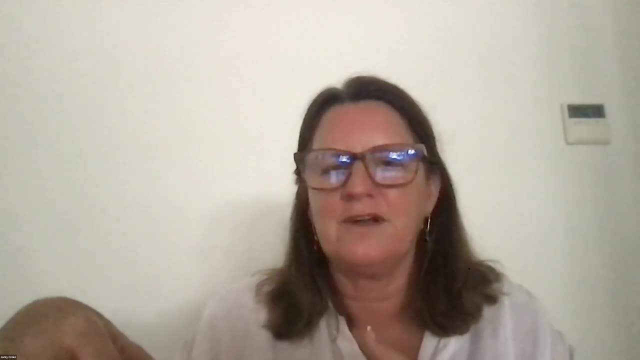 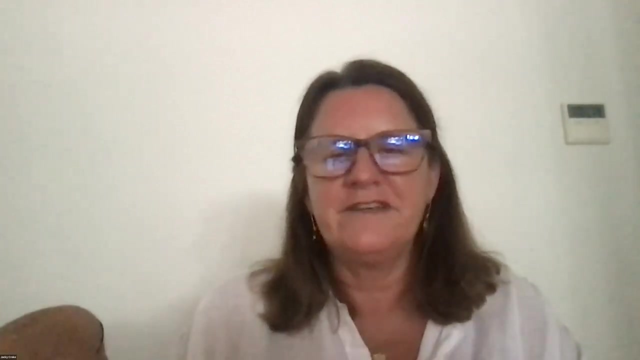 one in 1000, one in 5000. really, that's the crux of the problem. they well, they are managing for extreme events, but if we can go from a one in 5000 to a one in 90, just basically in two years, i think. 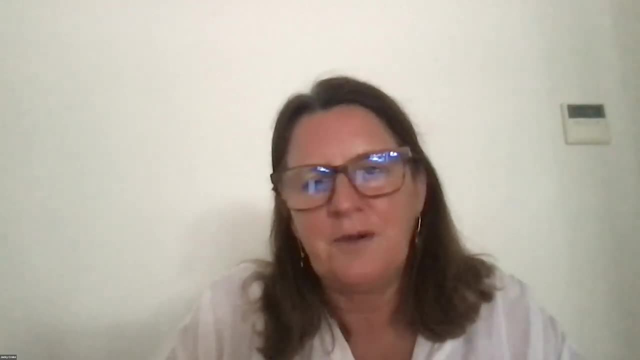 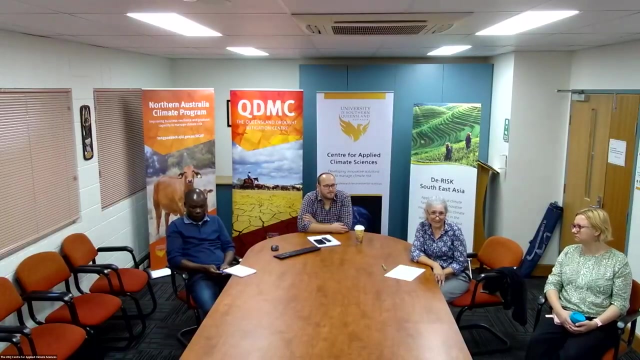 really that's fundamentally what the problem is. so they are aware of it. it's not that they're not managing that risk. no, it's it's. it's obviously a challenge. yeah, no, definitely it is a challenge for them and and really, you know the the only way that we can extend that. 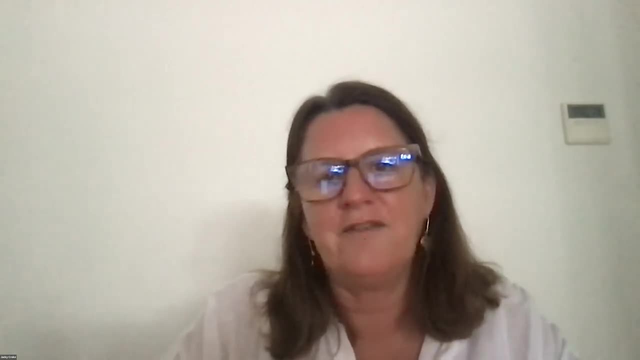 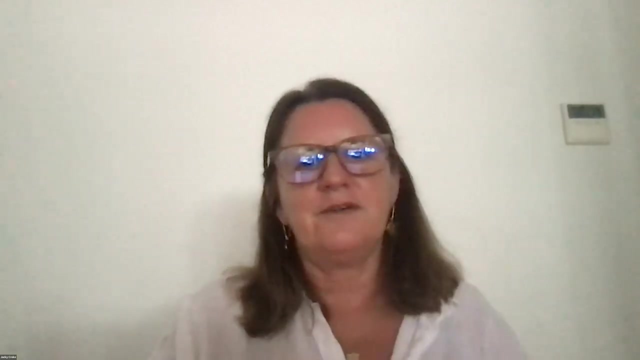 record is through paleoclimate data. you know we don't have another way, and i guess it's always been a little bit confusing for me why. you know a lot of people talk to me about accuracy and uncertainty when in fact, the historical record that we have is not accurate. it's recorded, it's. 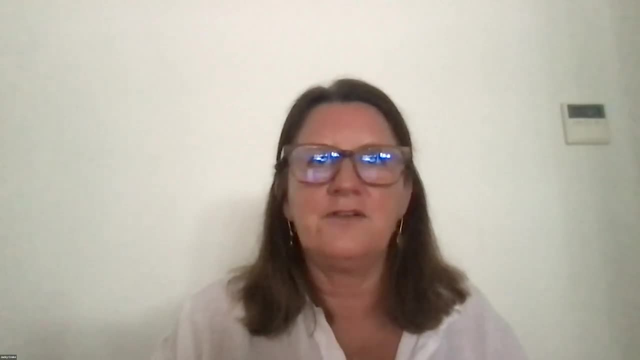 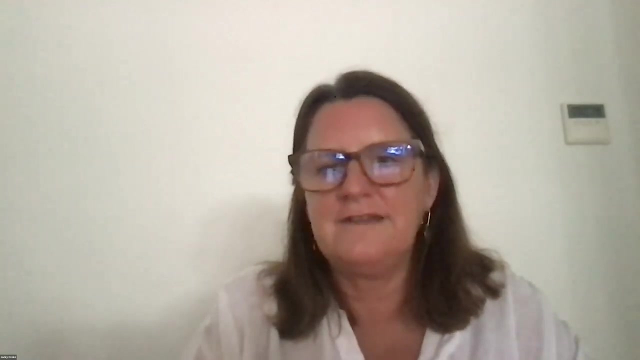 not accurate, um, but there is sort of a lot of focus really on uncertainty. that's why we went with the bayesian approach, because the uncertainty is is modeled into those reconstructions. so you know, sure there is uncertainty and you can see that once you go past 1600, for example, that uncertainty 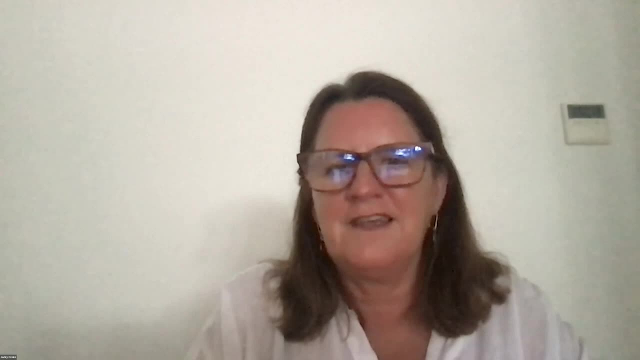 actually increases, but the extent to which that influences the output from a water resource model, it's marginal. it really is relative to that historic period because, like, do we genuinely feel that you know the data that we captured in 2022 is accurate? i mean, we've recorded it, but it's. 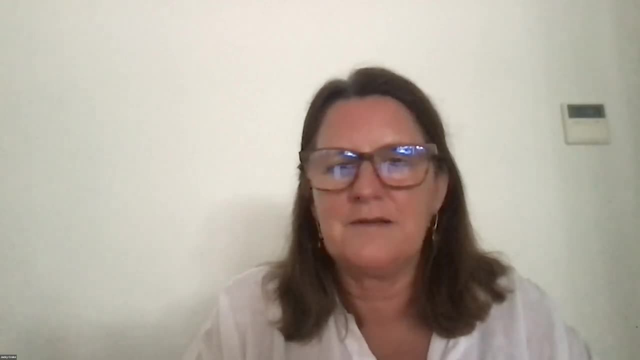 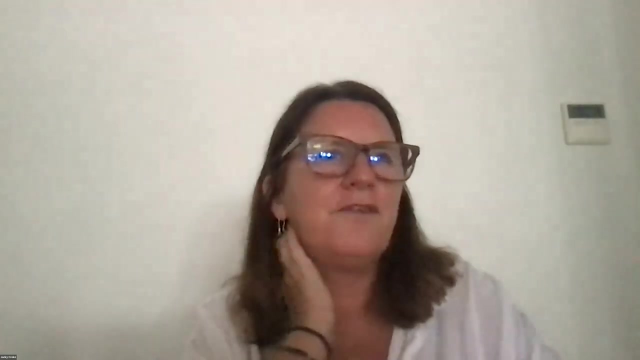 not accurate. most of the gauges would have been lost, i suspect. but um, so yeah, it's about the communication of some of that perception, i think so. are you involved in similar work in europe because there's been serious flooding? yeah, definitely. um, i'm involved in a couple of projects of water.